of your attention. So I'm going to explain only those things I think are the most worthy of your attention. So I'm going to explain only those things I think are the most worthy of your attention. So I'm going to explain only those things I think are the most worthy of remembering. 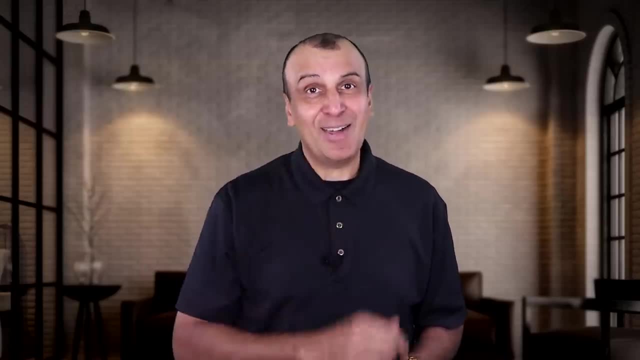 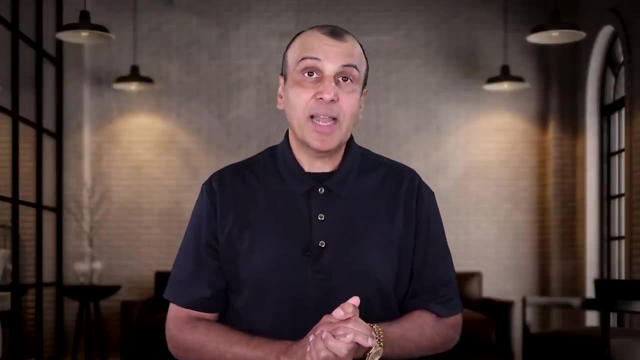 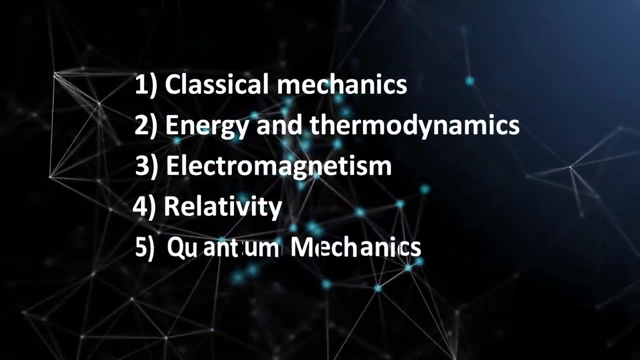 in all of physics That's coming up right now. There are five broad areas of physics that I think you should know a little bit about: Classical mechanics, energy and thermodynamics, electromagnetism, relativity and quantum mechanics. Classical mechanics is probably the most pertinent to your everyday experience. Here we 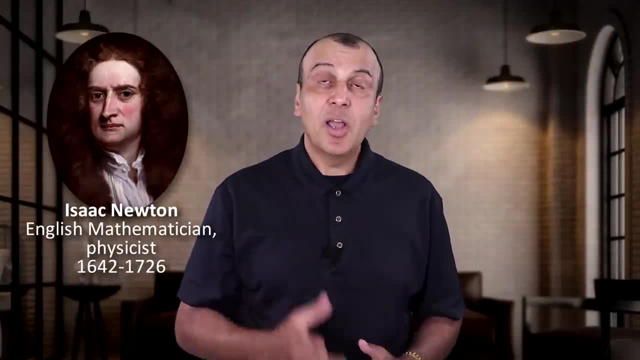 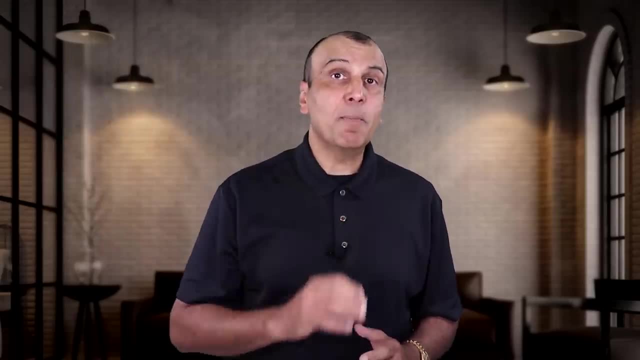 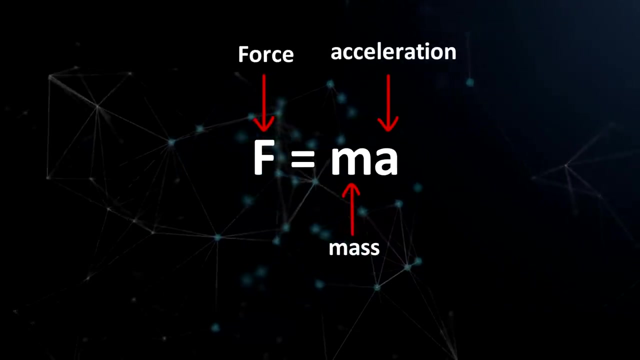 have to introduce the father of classical mechanics, Isaac Newton, arguably the greatest scientist of all time. There are two main concepts worthy of remembering. The first is embodied in Newton's second law: Force equals mass times acceleration. This is a deceptively simple equation that has 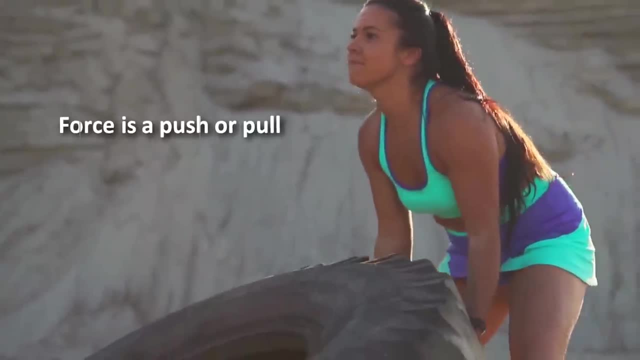 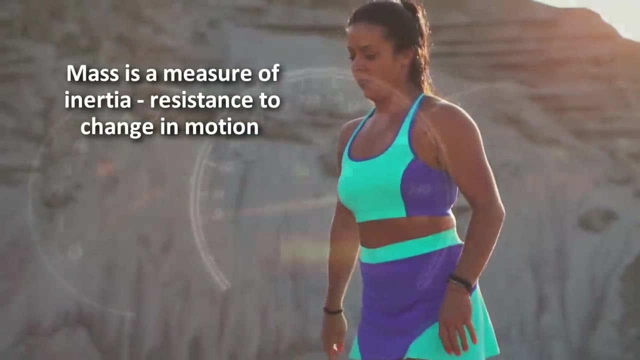 some huge ramifications. Force in classical physics just means a push or pull. Mass is a measure of inertia, how much something doesn't want to change in motion. Acceleration is how rapidly your velocity is changing. Acceleration is how rapidly your velocity is changing If you 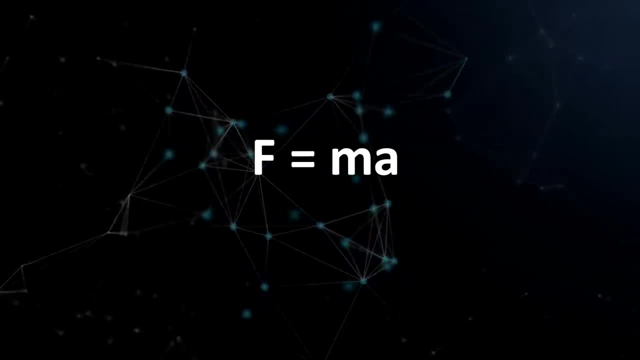 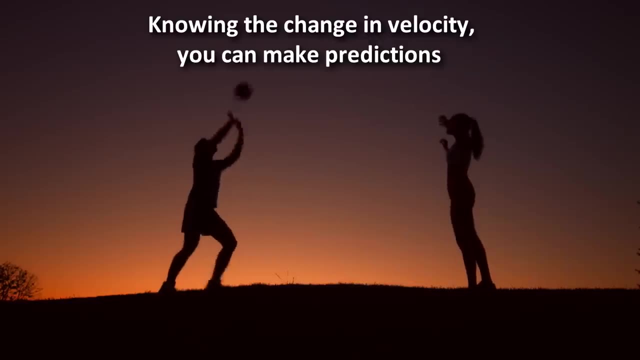 apply a force to a fixed mass, it tells you how much acceleration you will get And knowing acceleration, which is the change in velocity, you can make predictions like where an object will be at a certain time and space. So with this simple formula, for example, I can predict: 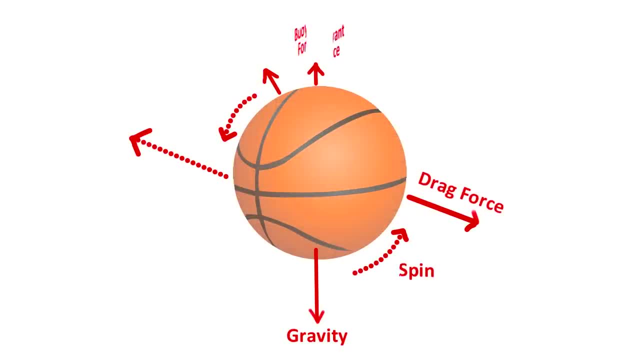 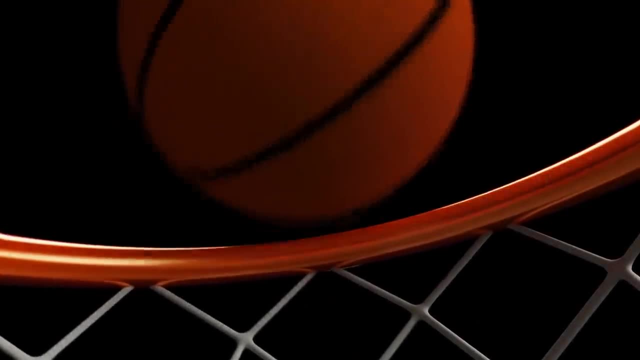 exactly where this basketball is and where it's going. If I know all the forces acting on it, including the friction of the air, which is also a force, I can predict exactly whether or not it will go through the hoop. This same formula can be used to determine how much reinforcement 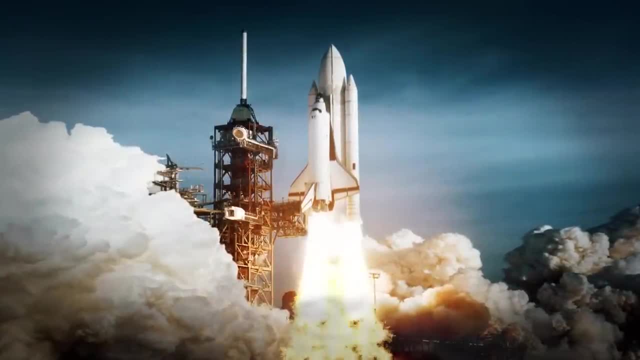 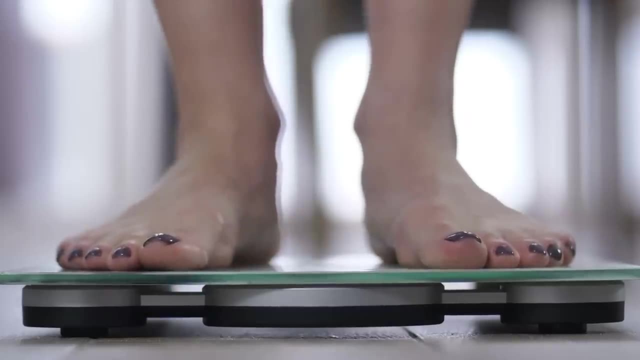 you would need to build a bridge, and how to calculate the lift of a rocket. It's an extremely powerful equation. Force is not a material thing. It is a measure of interaction. Your body does not have a force, It has a mass. Your weight is the force your body exerts on the ground. Technically, 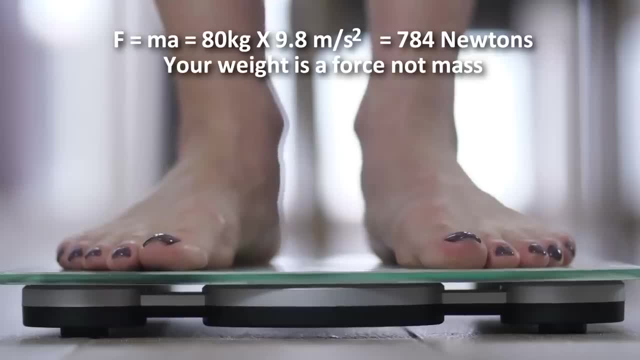 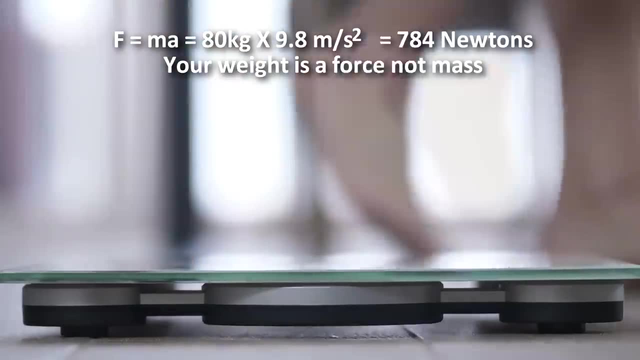 you don't weigh 80 kilograms, because that's your mass. You should be saying you weigh 784 newtons, which is your mass times the acceleration of gravity on earth: 9.8 meters per second squared. To give you an idea of scale, one newton of force. 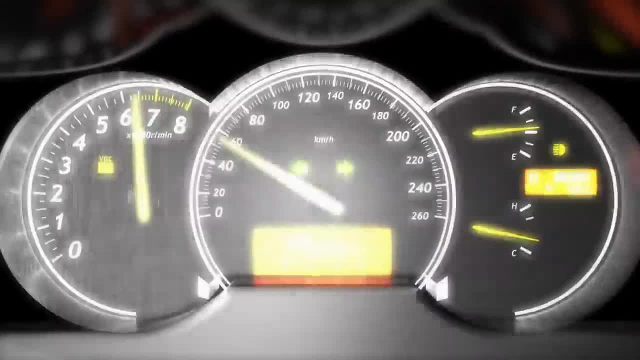 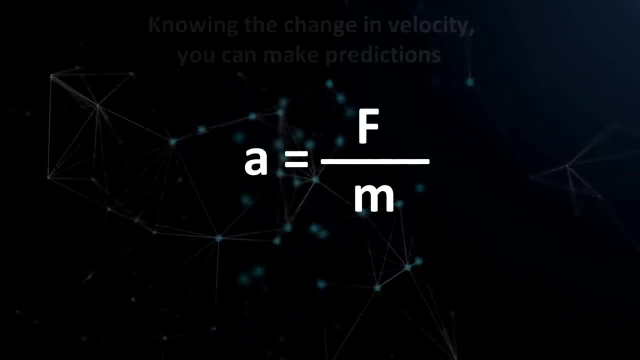 Acceleration is how rapidly your velocity is changing. If you apply a force to a fixed mass, it tells you how much acceleration you will get And knowing acceleration, which is the change in velocity, you can make predictions like where an object will be at a certain time. 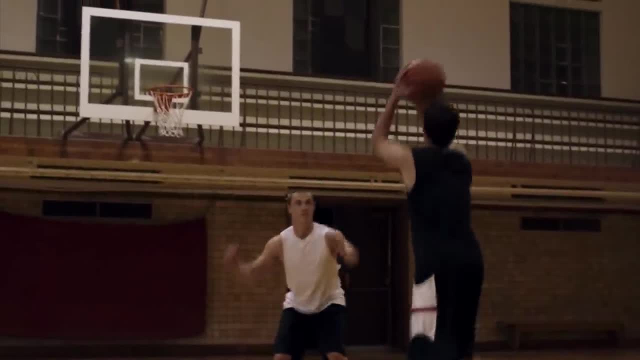 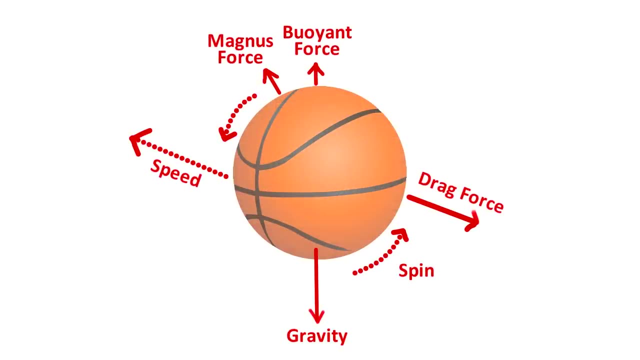 and space. So with this simple formula, for example, I can predict exactly where this basketball is and where it's going. If I know all the forces acting on it, including the friction of the air, which is also a force, I can predict exactly whether or not it will go through the hoop. 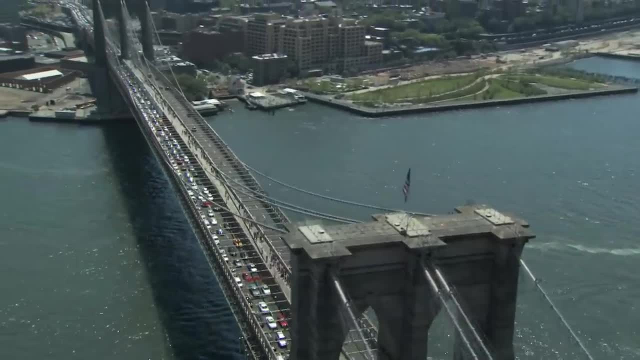 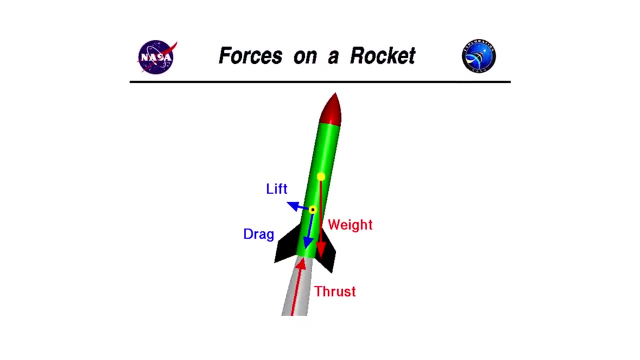 This same formula can be used to determine how much reinforcement you would need to build a bridge and how to calculate the lift of a rocket. It's an extremely powerful equation. Force is not a material thing. It is a measure of interaction. Your body does not have a force. 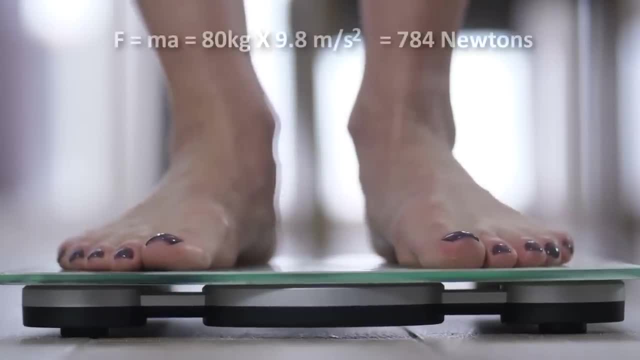 it has a mass. Your weight is the force your body exerts on the ground. Technically, you don't weigh 80 kilograms because that's your mass. You should be saying you weigh 784 newtons, which is your mass, times the acceleration of gravity on earth: 9.8 meters per second squared. 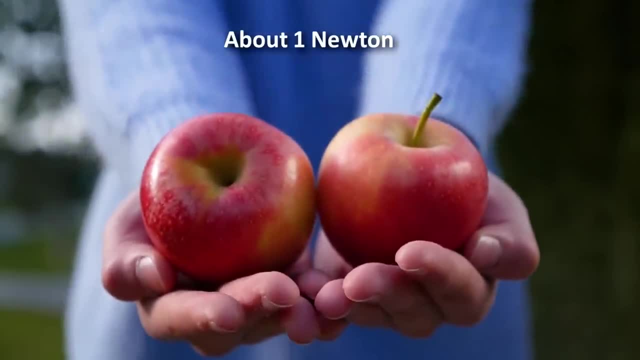 To give you an idea of scale, one newton of force is equivalent to the force you lift on the ground. This is the force you lift on the ground. This is the force you lift on the ground. You would feel on your palm if you were holding a small apple. The second equation, also from: 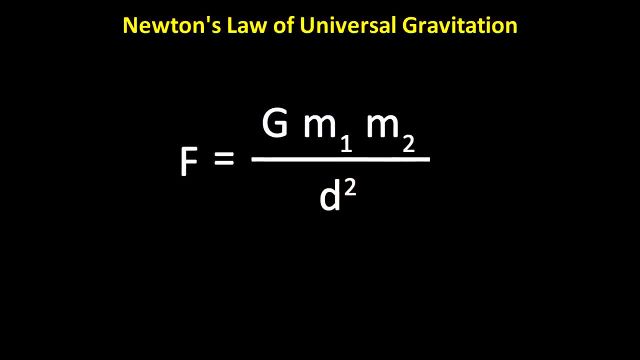 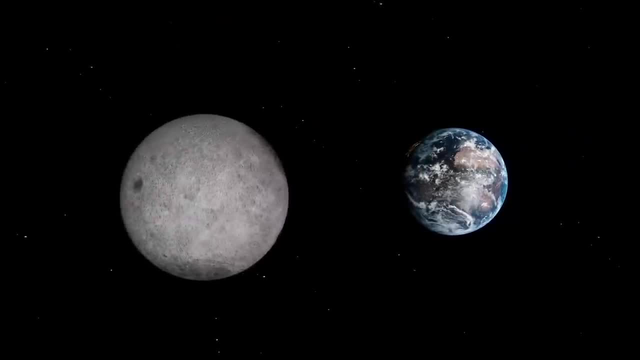 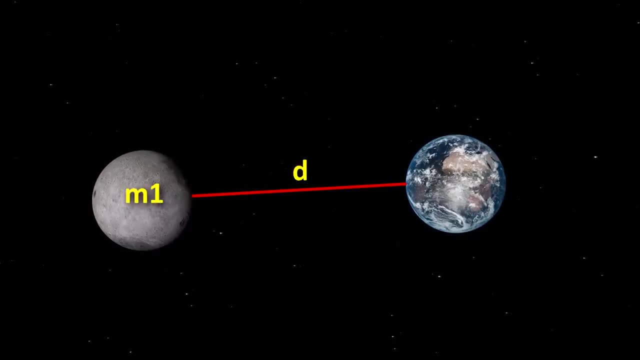 Newton is the law of universal gravitation. It allows us to determine the motion of heavenly bodies like the moon orbiting the earth or planets orbiting stars. It basically says that the gravitational attraction between two bodies is the product of their masses divided by the distance. 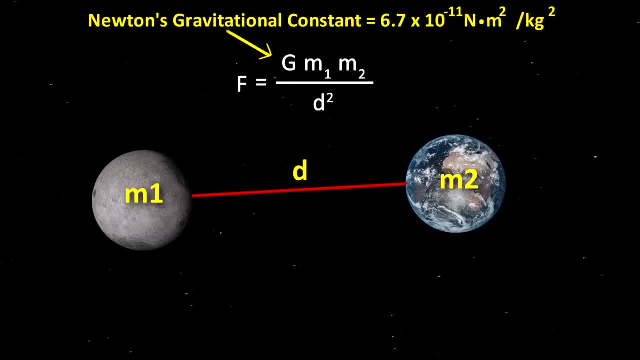 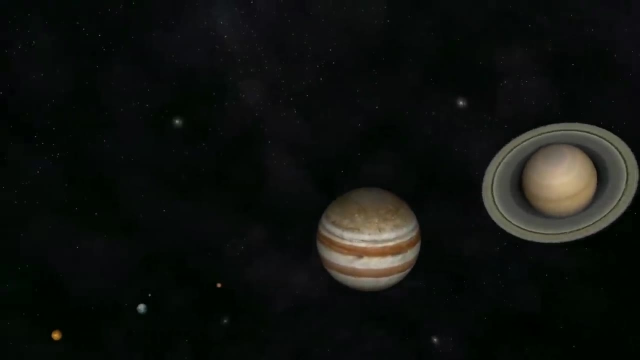 between them squared times a constant called Newton's gravitational constant. It tells you that the gravitational attraction diminishes rapidly as objects move apart, because it's proportional to the inverse of distance squared. This was a revelation when Newton formulated it, because it explained mathematically the movement of all heavenly bodies. It still works well today. 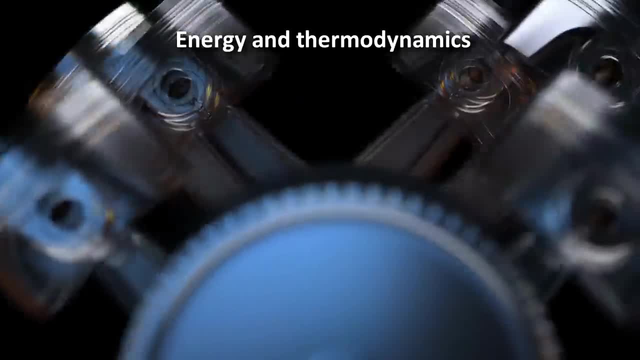 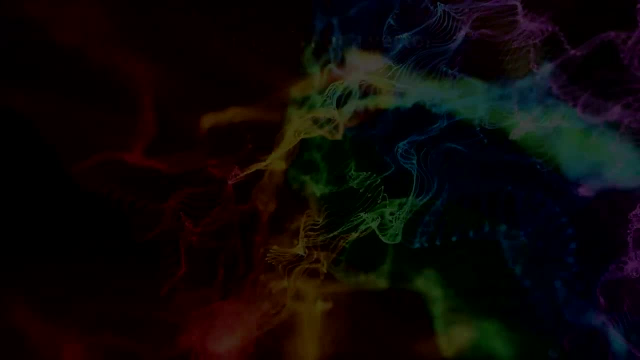 The ideas around energy came about a hundred years after Newton. It may be the most important idea in physics. Energy is not a vector like force or momentum. It doesn't have direction, but it is a number. Work is closely related to energy. It has the same. 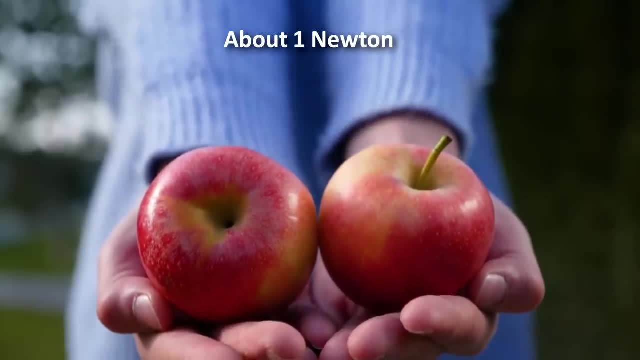 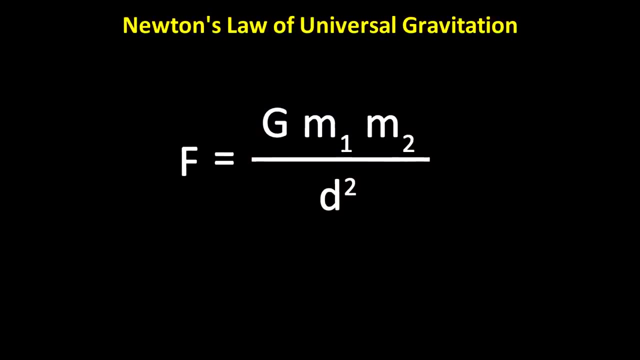 is equivalent to the force you would feel on your palm if you were holding a small apple. The second equation, also from newton, is the law of universal gravitation. It allows us to determine the motion of heavenly bodies like the moon orbiting the earth or planets orbiting stars. 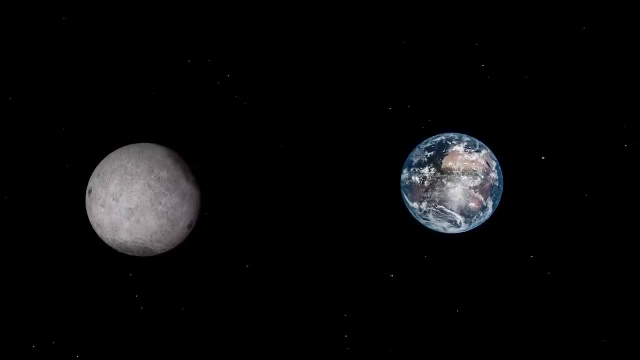 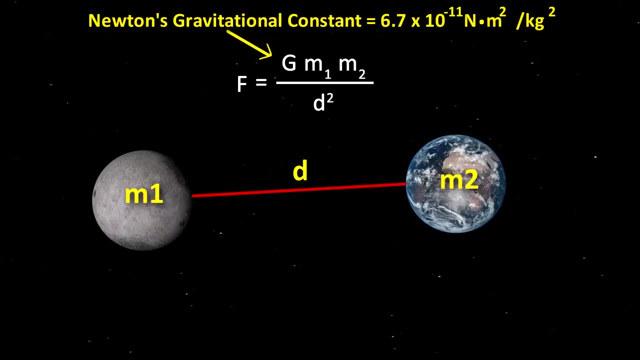 It basically says that the gravitational attraction between two bodies is the product of their masses divided by the distance between them squared times a constant called newton's gravitational constant. It tells you that the gravitational attraction diminishes rapidly as objects move apart, because it is proportional to the inverse of distance squared. This was a revelation when newton 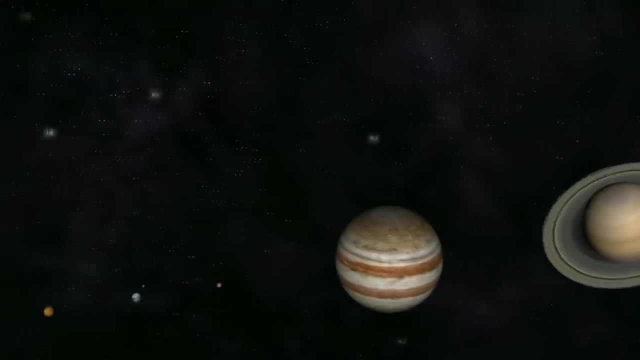 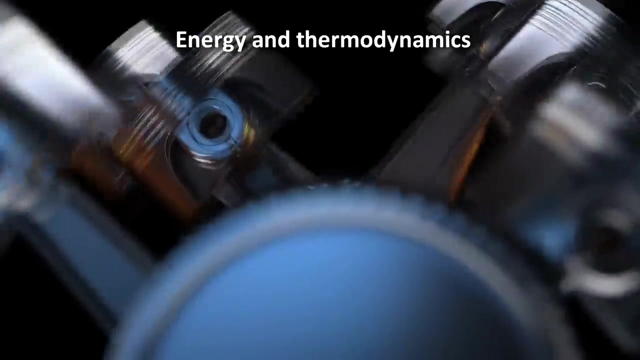 formulated it because it explained mathematically the movement of all heavenly bodies. It still works well today. The ideas around energy came about 100 years after newton. It may be the most important idea in physics. Energy is not a vector like force or momentum. It doesn't have direction, but it is. a number. Work is closely related to it. It is not a vector like force or momentum. It is not a vector like force or momentum. It is a number. Work is closely related to it. It is a number. Work is closely related to it. It is a number. Work is closely related to it. It is a number. Work is closely related to. 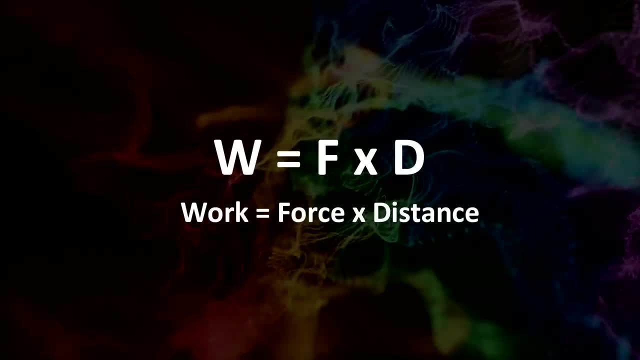 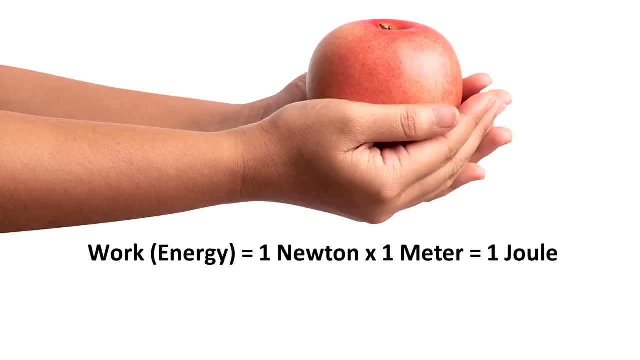 energy It has the same units. Work is force times distance traveled. One newton times one meter is one joule. If you lift a small apple, one meter, that takes one joule of energy. or work- Energy is really a measure of how much work you can do. Work is simply transferring energy from 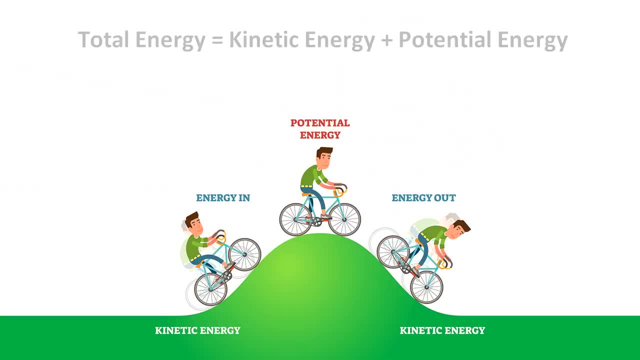 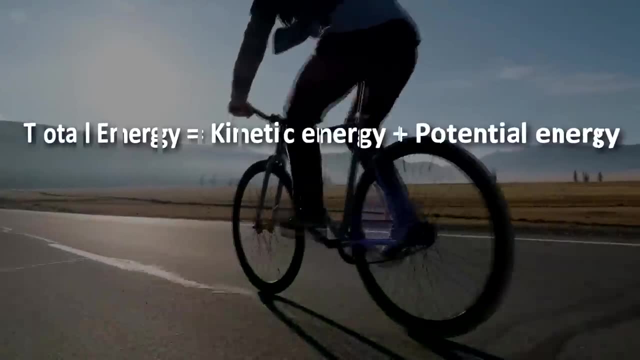 one form to another. Energy for most objects consists of kinetic energy plus potential energy. Kinetic energy is the energy of motion. It is expressed as one half times the mass times velocity. Energy is the energy of motion. It is expressed as one half times the mass times velocity. 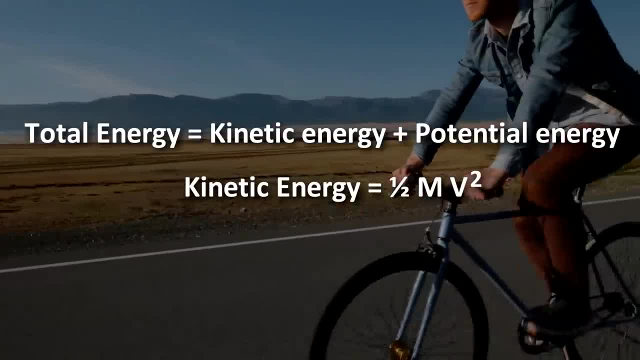 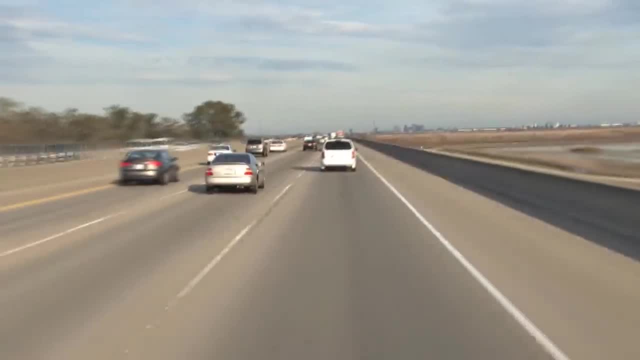 Energy is the energy of motion. It is expressed as one half times the mass times velocity. The more mass you have and the more velocity you have, the more energy you have. Velocity makes a bigger difference in energy than mass, Going from 80 miles per hour to 60. 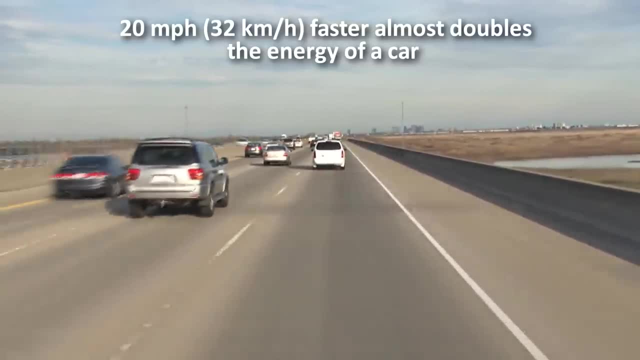 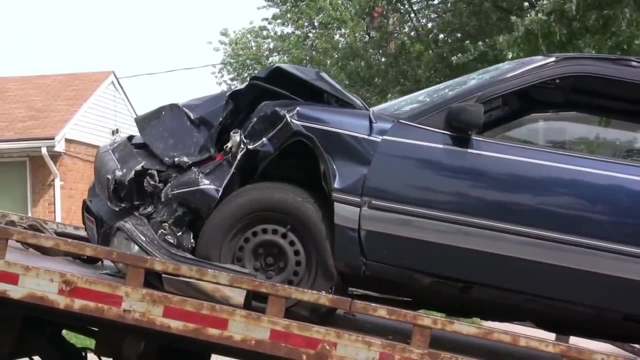 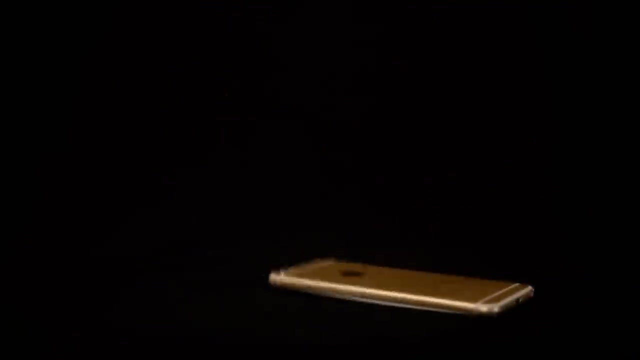 miles per hour reduces your car's energy by almost 50%, which means that in an accident, you have a much higher chance to survive going 20 miles per hour slower. If you are carrying your phone and you accidentally drop it from rest onto concrete, your phone is probably going to get damaged. But where does the energy come from? 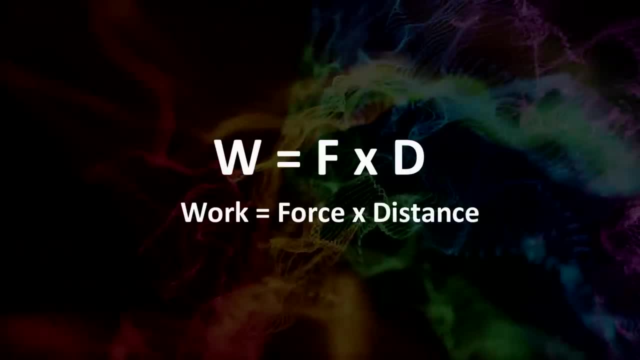 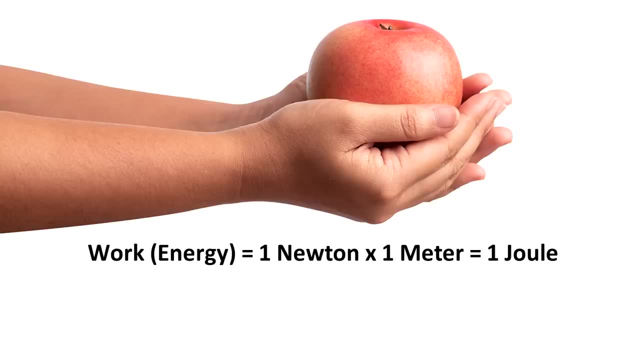 units. Work is force times, distance traveled, One newton times. one meter is one joule. If you lift a small apple, one meter that takes one joule of energy. or work: Energy is really a measure of how much work you can do. Work is simply transferring energy from one form to another. 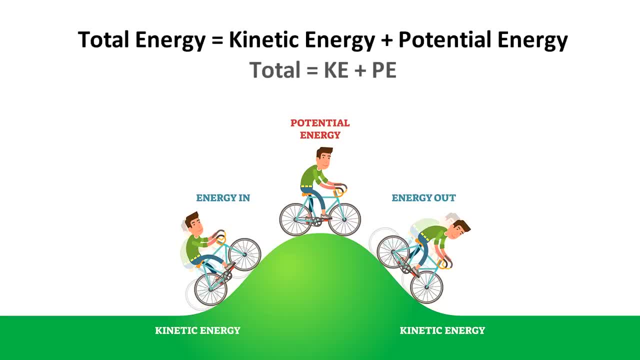 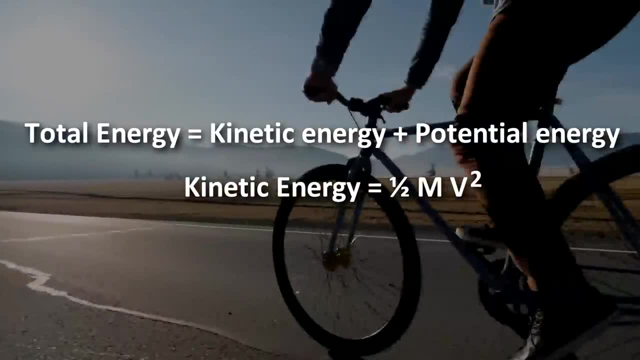 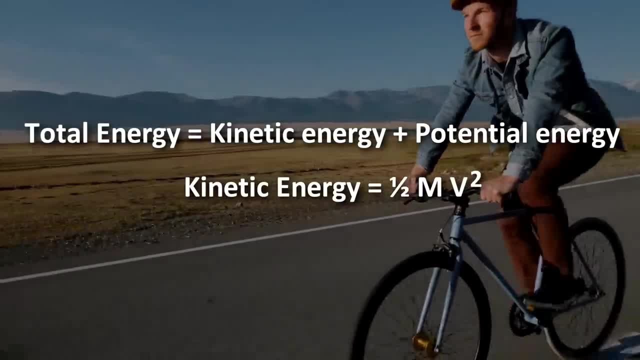 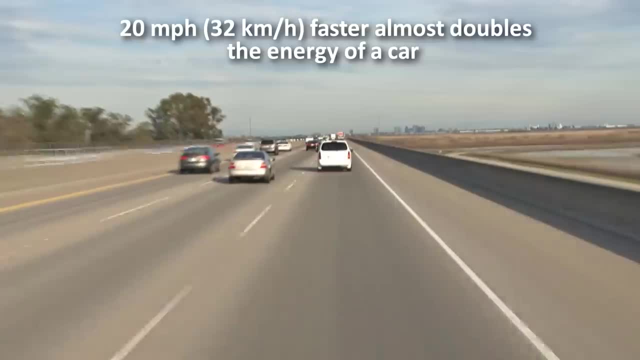 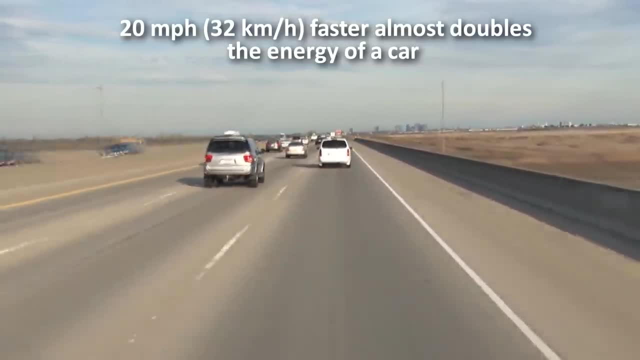 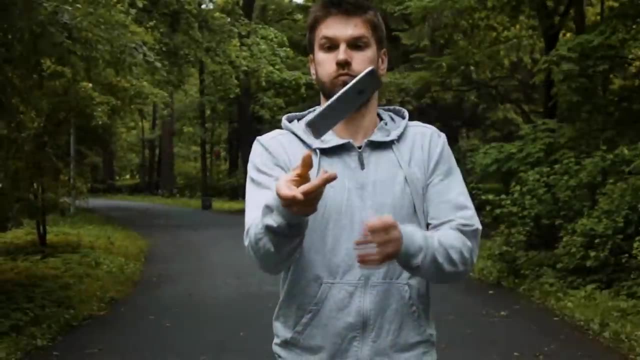 car's energy by almost 50 percent, which means that in an accident you have a much higher chance to survive going 20 miles per hour slower. If you're carrying your phone and you accidentally drop it from rest onto concrete, your phone is probably going to get damaged. 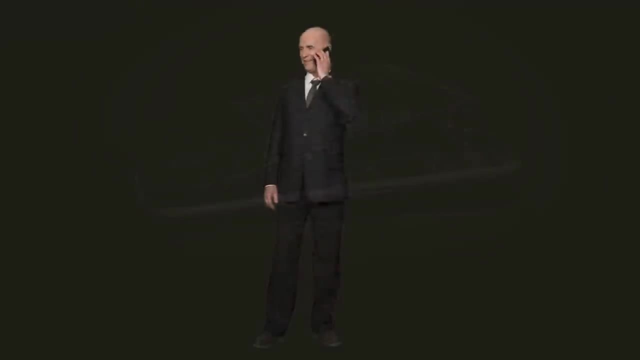 But where did the energy come from to damage it? The phone had what is called potential gravitational energy. when you were holding it near your ear, The potential energy was converted to kinetic energy as it fell. Gravitational potential energy is expressed as mass times the gravitational acceleration, times the height. 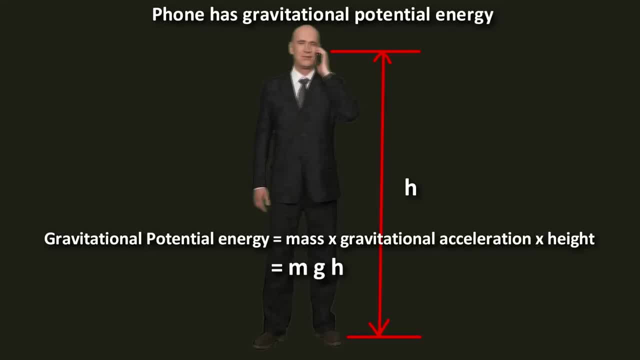 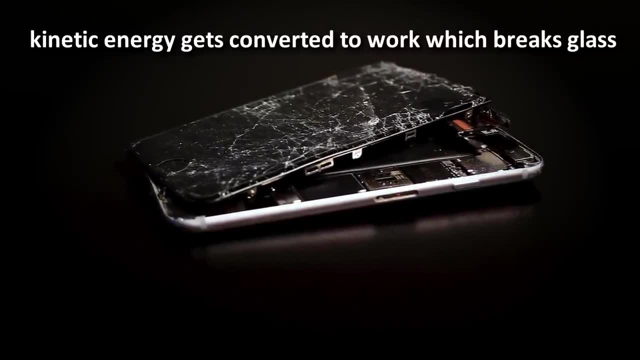 This is really another way to express force: times, distance or work. This potential energy gets converted to work or a force acting on the glass which breaks it when the phone hits the floor. So the total energy of an object is both kinetic energy plus potential energy Potential. 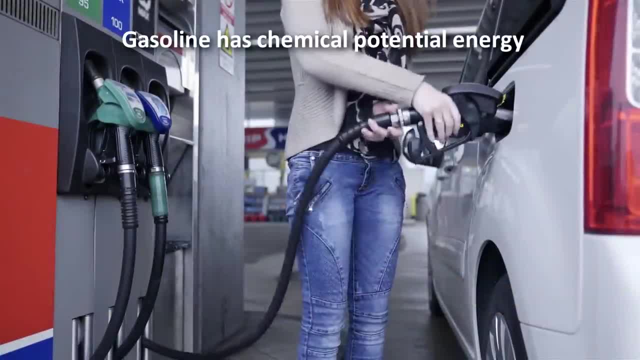 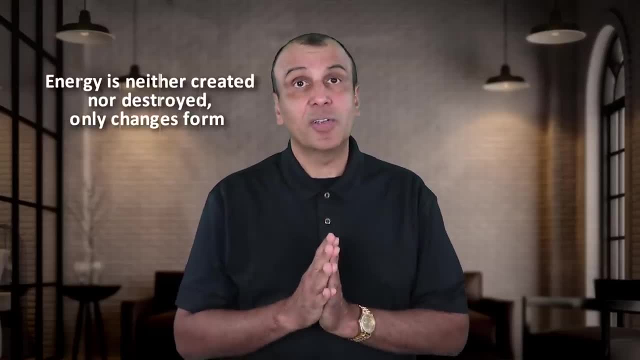 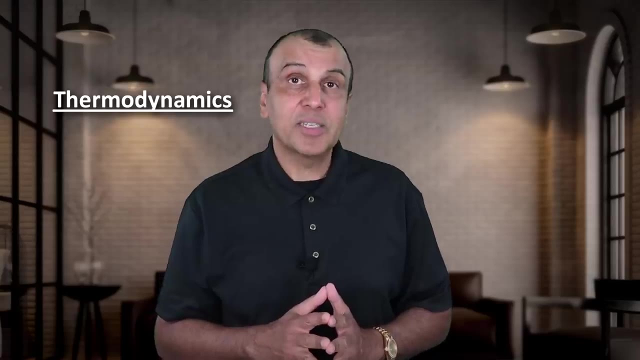 energy can take many forms. Gasoline or petrol, for example, has chemical potential energy. The biggest thing you should remember about energy is that it's always conserved. It's not created or destroyed. It only changes form. Now, talk about energy leads naturally to thermodynamics, which is 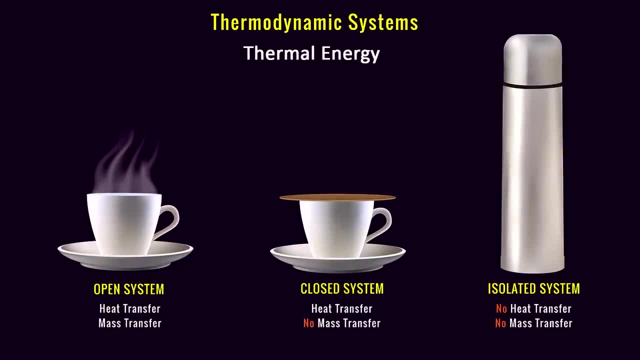 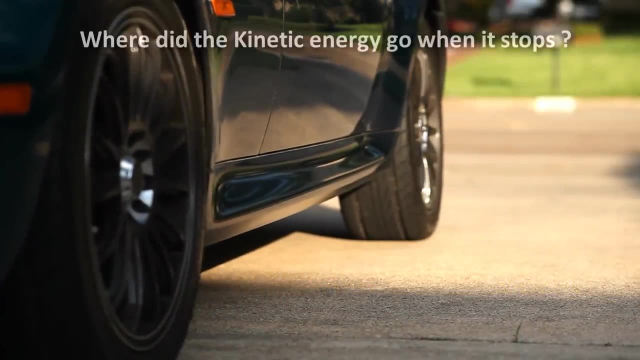 the study of work, heat and energy in a system. The biggest concept worthy of remembering is flow of heat. We defined energy as how much work you could do. But another form of energy is thermal energy. If a car is moving and you apply the brakes, the kinetic energy of the car becomes zero. 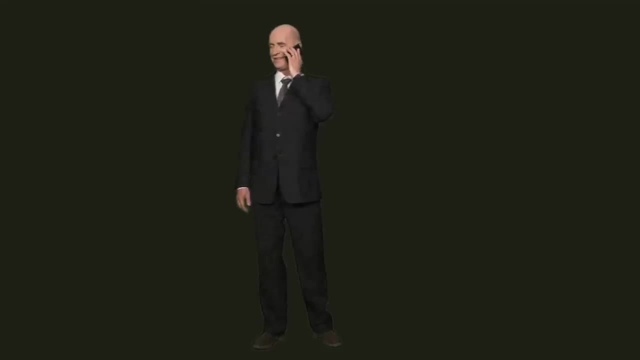 The phone had what is called potential gravitational energy. when you were holding it near your ear, The potential energy was converted to kinetic energy as it fell. Gravitational potential energy is expressed as mass times the gravitational acceleration times the height. This is really another way to express force times distance or work. 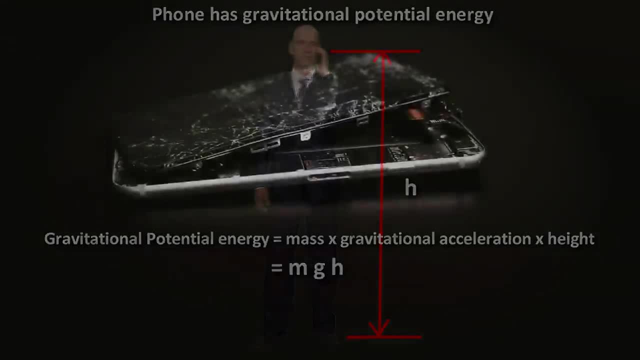 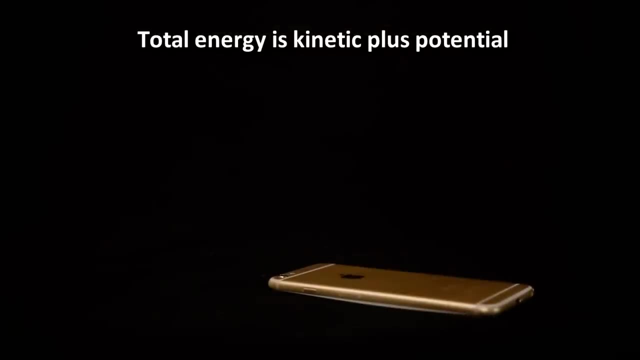 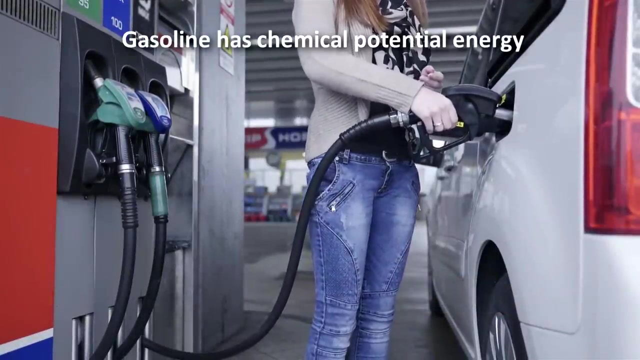 This potential energy gets converted to work or a force acting on the glass, which breaks it when the phone hits the floor. So the total energy of an object is both kinetic energy plus potential energy. Potential energy can take many forms. Gasoline or petrol, for example, has chemical potential energy. 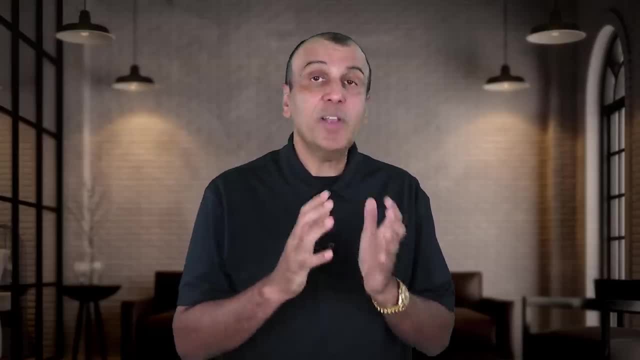 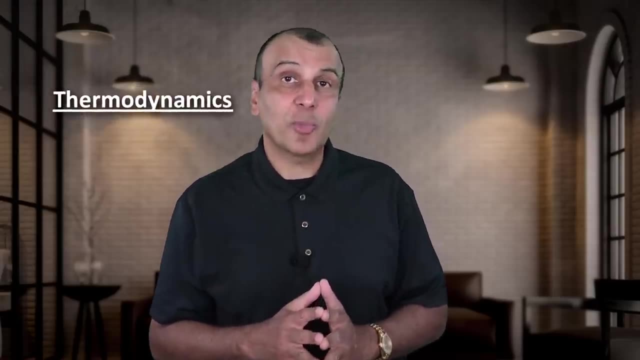 The biggest thing you should remember about energy is that it is always conserved. It is not created or destroyed, it only changes form. Now talk about energy leads naturally to thermodynamics, which is the study of work, heat and energy in a system. 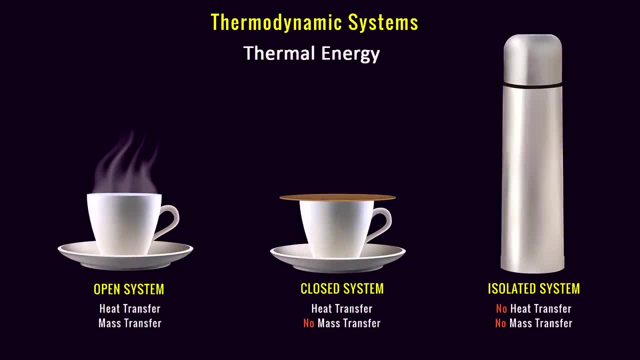 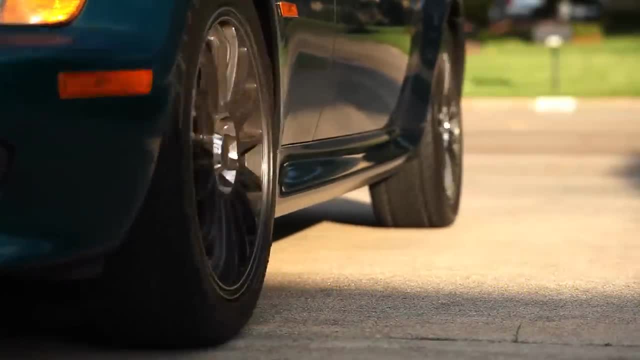 The biggest concept worthy of remembering is flow of heat. We defined energy as how much work you could do. The second form of energy is thermal energy. If a car is moving and you apply the brakes, the kinetic energy of the car becomes zero. 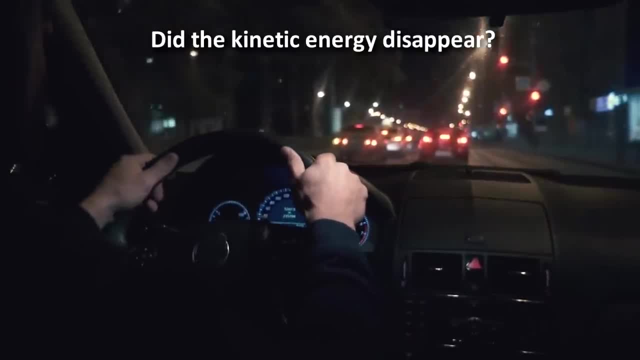 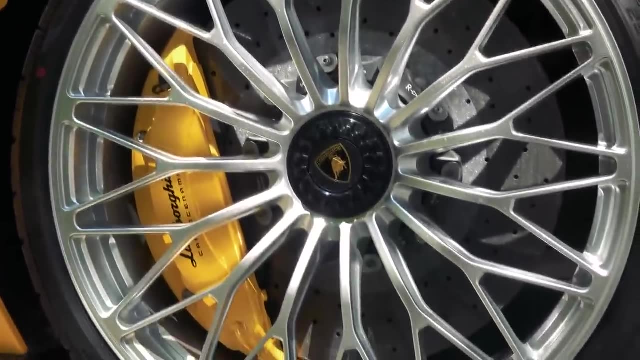 Where did that energy go? It didn't go to gravitational potential energy and it's not stored in the car somewhere Did it disappear? No, it was converted to thermal energy created by friction of the car's brakes. Heat is a flow of thermal energy from one object to another. 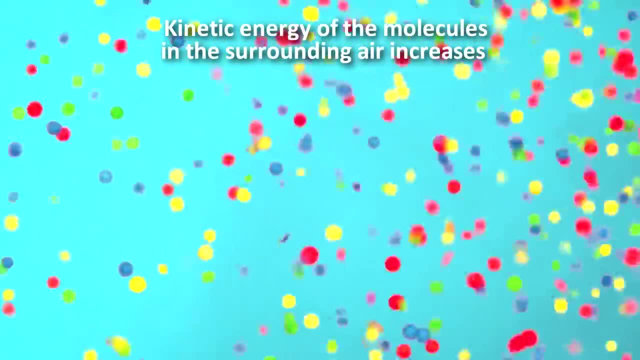 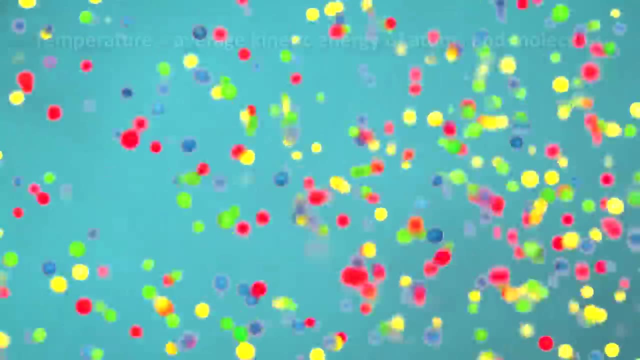 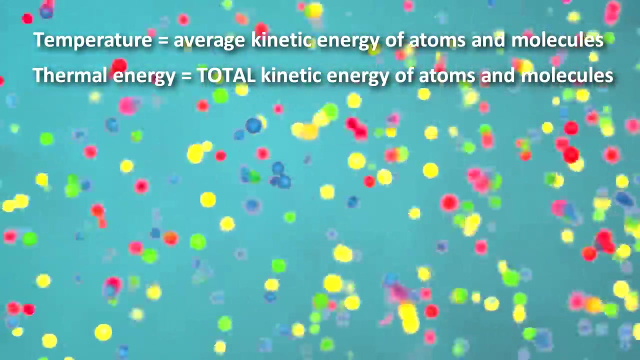 Thermal energy created by the brakes raises the kinetic energy or movement of molecules In the air. this results in a temperature increase of the surrounding air. This is ultimately where the kinetic energy of your car ends up after you come to a stop. The temperature of a system is the average kinetic energy of atoms in the system. 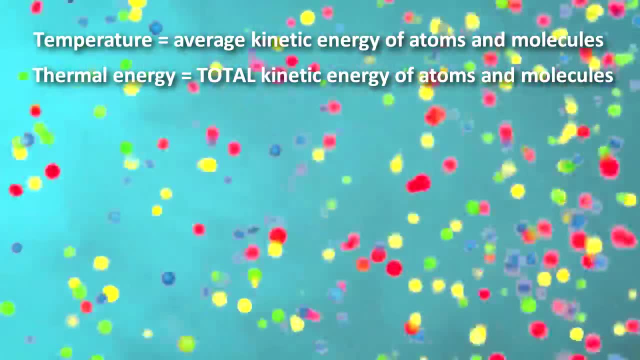 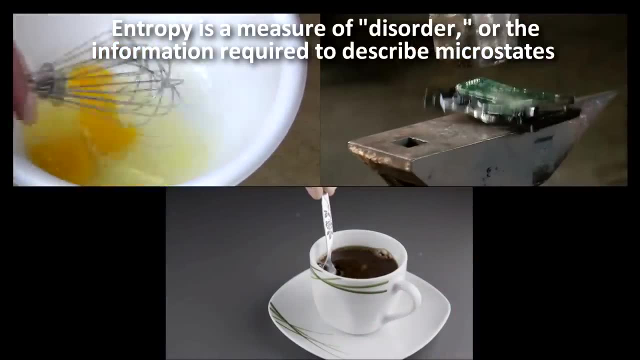 Thermal energy is the total amount of kinetic energy of atoms in the system. Another concept in thermodynamics is the idea of entropy. Entropy is a measure of disorder, but more accurately, it is a measure of the information that is present in the system. 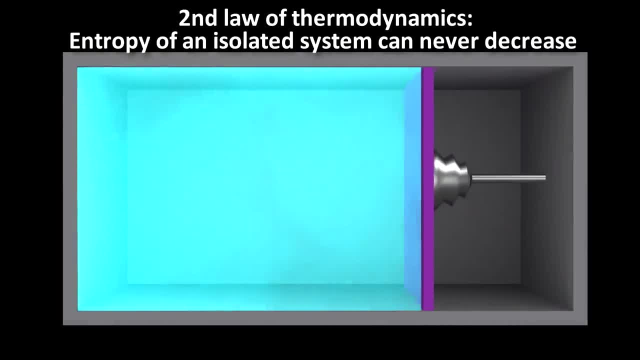 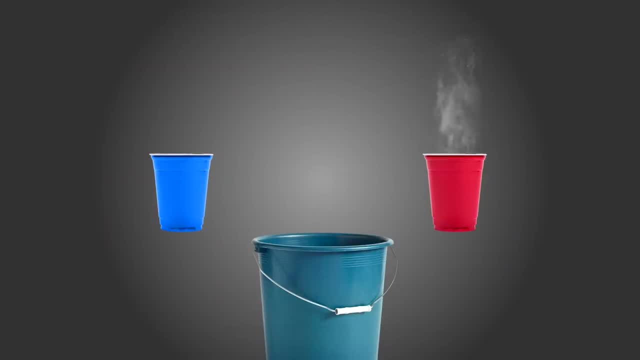 The second law of thermodynamics states that the entropy of an isolated system can never decrease. If you put two liquids together in a bucket and one is very cool and the other is very hot, why can't you get it such that the cold part gets colder and the hot part gets hotter? 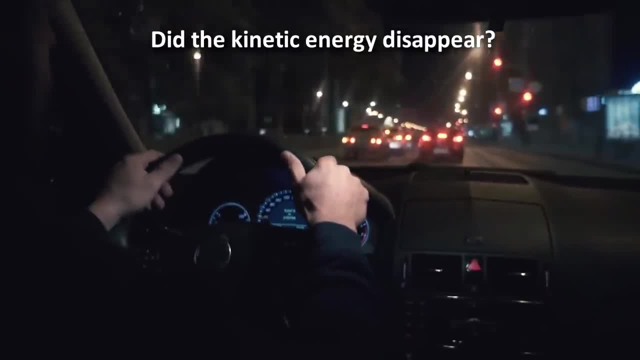 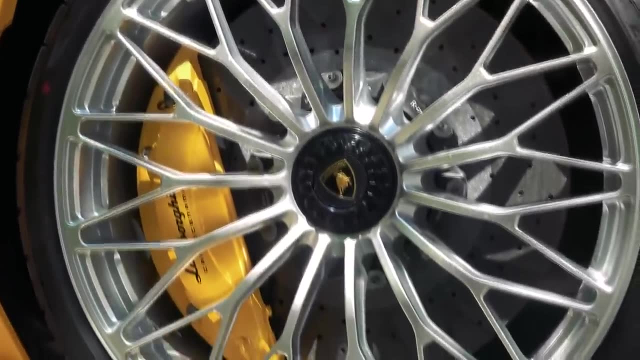 Where did that energy go? It didn't go to gravitational potential energy and it's not stored in the car somewhere. Did it disappear? No, It was converted to thermal energy created by friction of the car's brakes. Heat is a flow of thermal energy from one object to another. Thermal 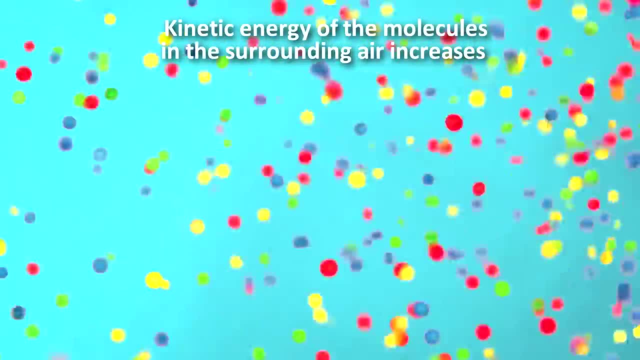 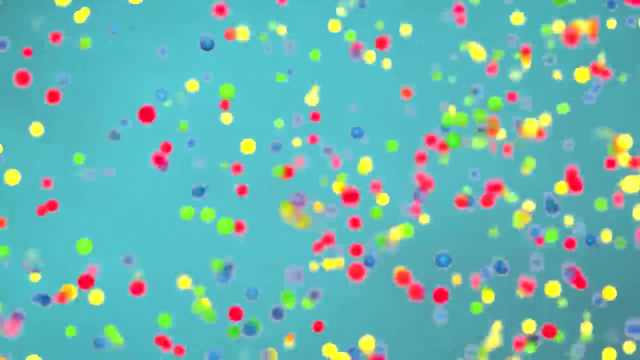 energy created by the brakes raises the kinetic energy or movement of molecules in the air. This results in a temperature increase of the surrounding air. This is ultimately where the kinetic energy of your car ends up. after you make a stop, The temperature of a system is the. 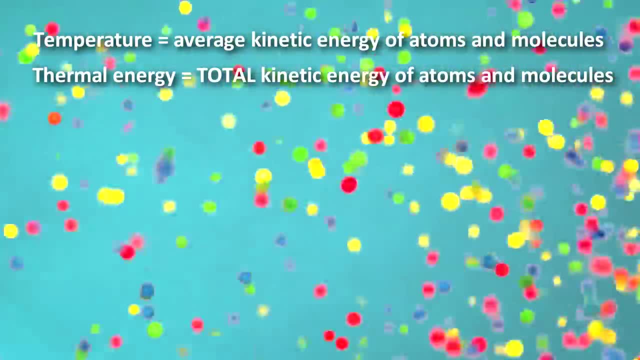 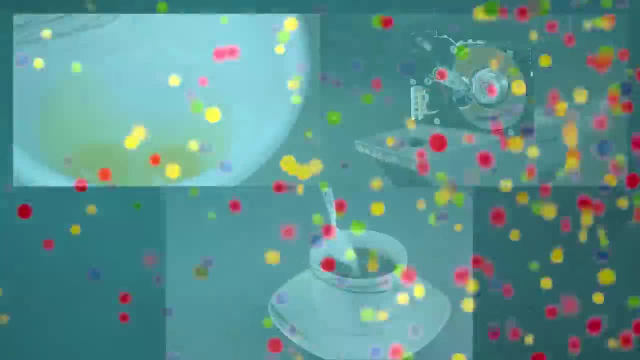 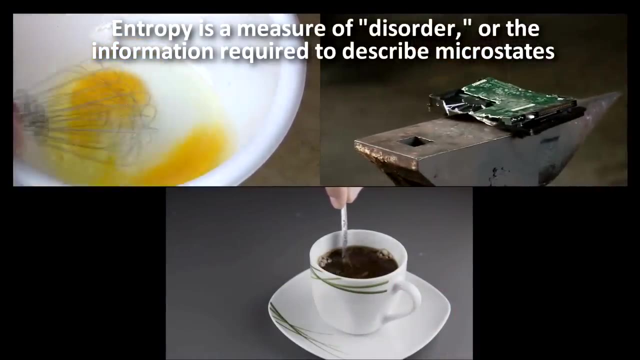 average kinetic energy of atoms in the system. Thermal energy is the total amount of kinetic energy of atoms in the system. Another concept in thermodynamics is the idea of entropy. Entropy is a measure of disorder, but more accurately it is a measure of the information. required – the energy dump and the future. In alloras, the temperature is equal to the energy resulting from having a star in the air. The energy voice recording is the expression of the energy decreasing thermal energy. This much accuracy almost nuoptly reduces a car or vehicle's power sharing. 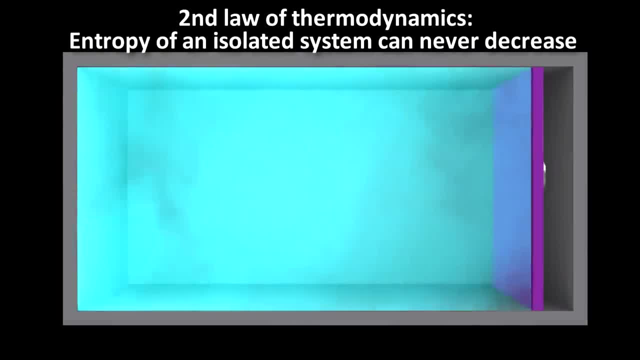 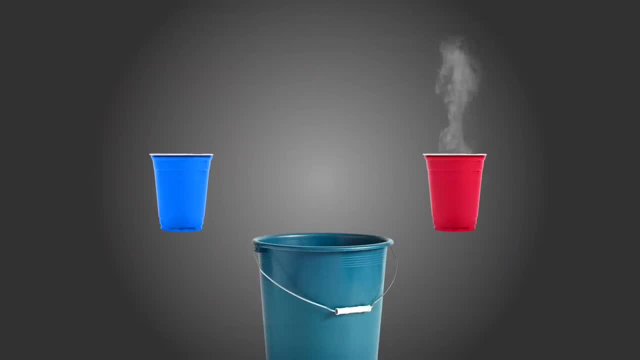 describe the microstates of a system. The second law of thermodynamics states that the entropy of an isolated system can never decrease. If you put two liquids together in a bucket and one is very cool and the other is very hot, why can't you get it such that the cold? 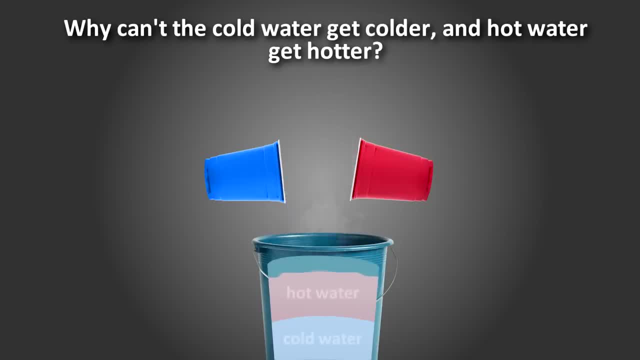 part gets colder and the hot part gets hotter, Energy could still be conserved because the decrease in thermal energy of the cold water could be offset by the increase in thermal energy of the hot water. The reason this does not happen is because of the second law. 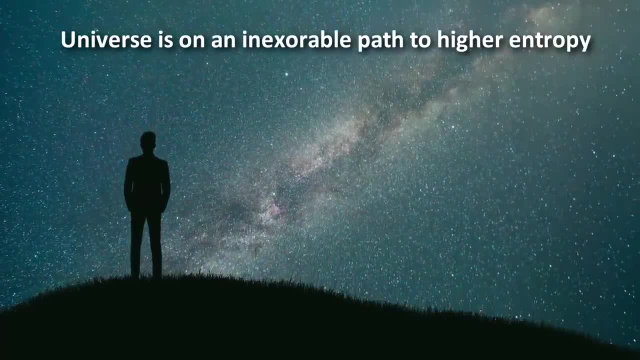 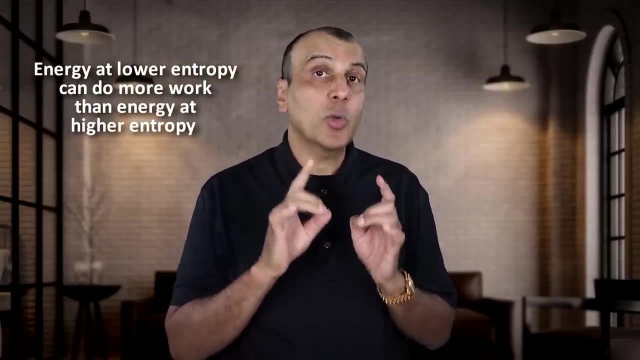 The universe is on an inexorable path to higher and higher entropy or more and more disorder. Practically, what this law tells us is that some energy is more useful for doing work than others. Energy at lower entropy can do more work than energy at higher entropy, For 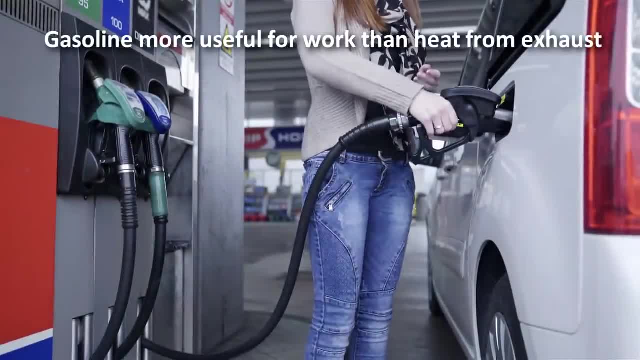 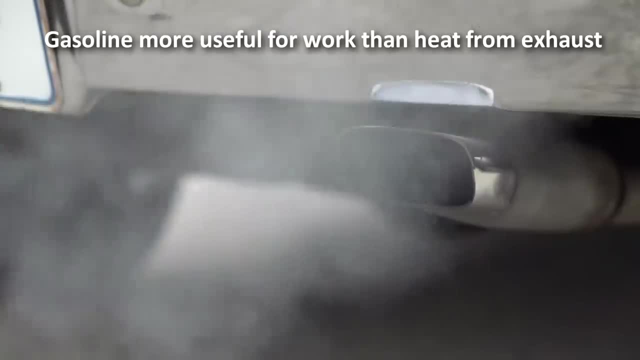 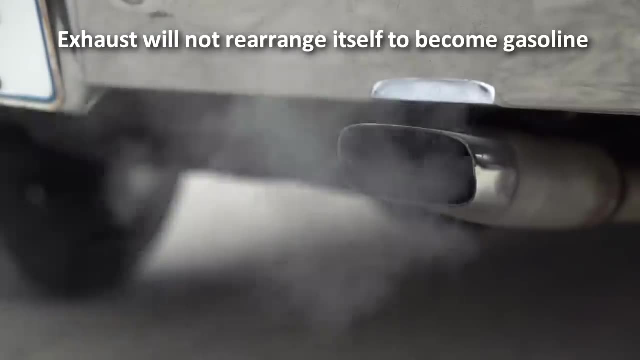 example, the energy stored in gasoline is more useful for doing work then the thermal energy that is disappeared from our life from the brakes of your car. An orderly energy is more useful than one that is less orderly. The heat and exhaust from the car will not spontaneously rearrange itself to become the 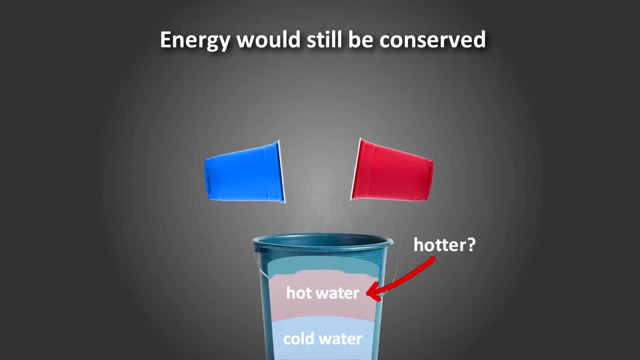 Energy could still be conserved, because the decrease in thermal energy of the cold water could be offset by the increase in thermal energy. So what's the answer? The answer is the thermal energy of the hot water. The reason this does not happen is because of the second law. 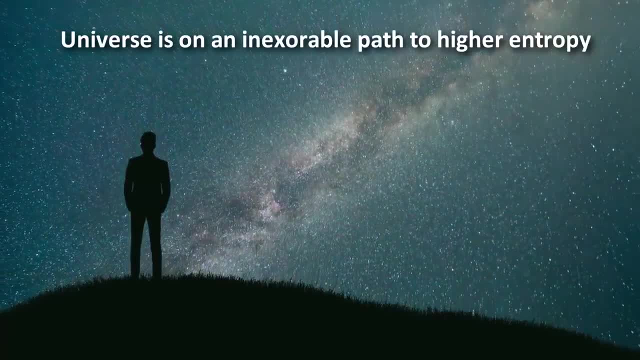 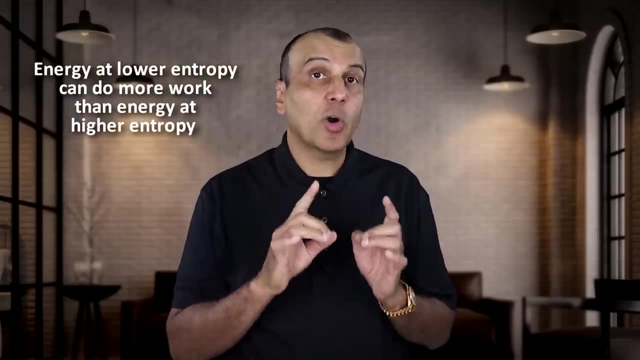 The universe is on an inexorable path to higher and higher entropy or more and more disorder. Practically, what this law tells us is that some energy is more useful for doing work than others. Energy at lower entropy can do more work than energy at higher entropy. 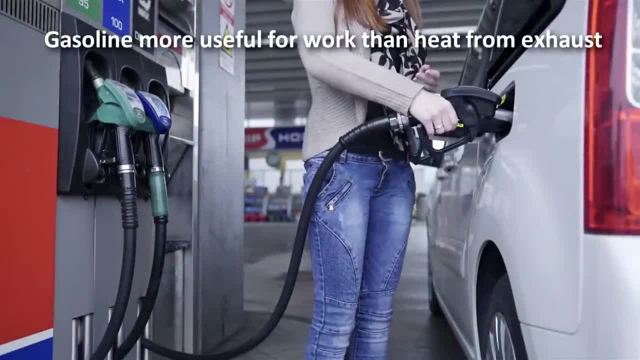 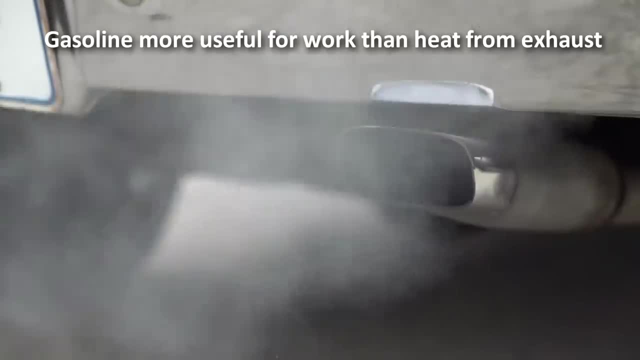 For example, the energy stored in gasoline is more useful for doing work than the thermal energy that is discharging. Energy stored in gasoline is more useful for doing work than the thermal energy that is dissipating from the brakes of your car. An orderly energy is more useful than one that is less orderly. 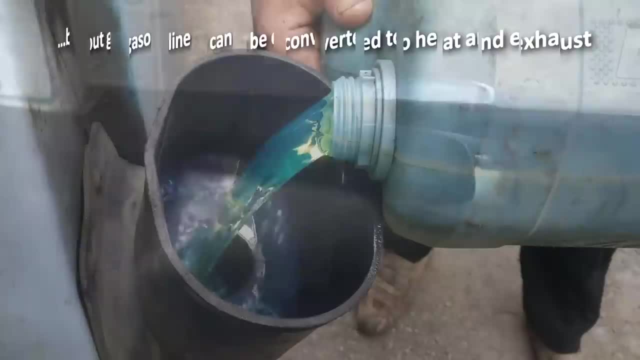 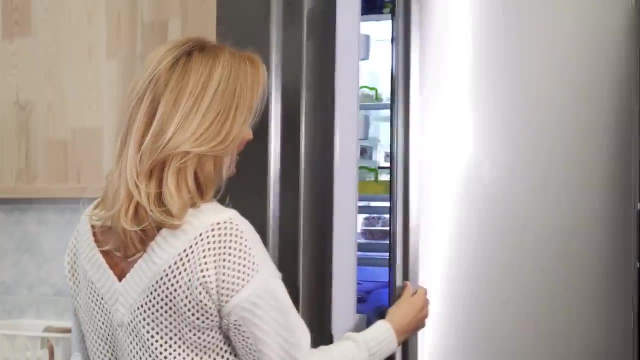 The heat and exhaust from the car will not spontaneously rearrange itself to become the gasoline, but gasoline can be converted to heat and exhaust. It's important to remember the words isolated system. If you put a glass of water in the freezer, it will decrease the entropy. 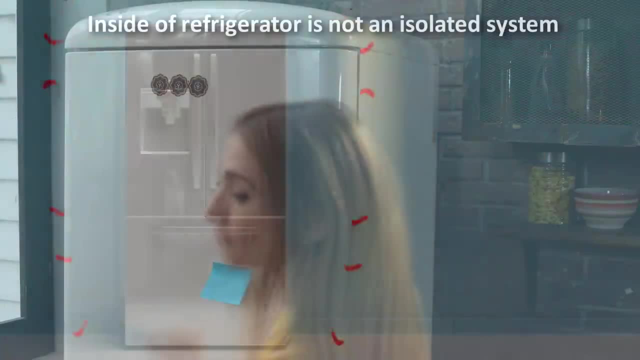 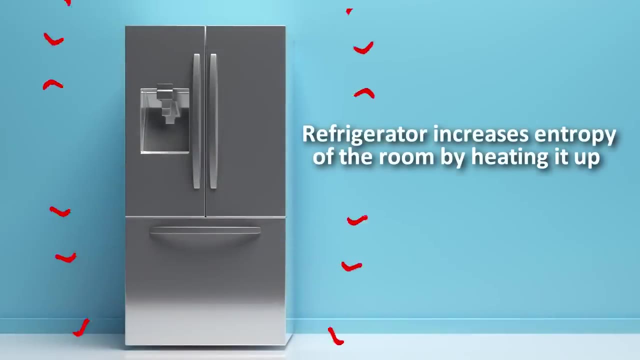 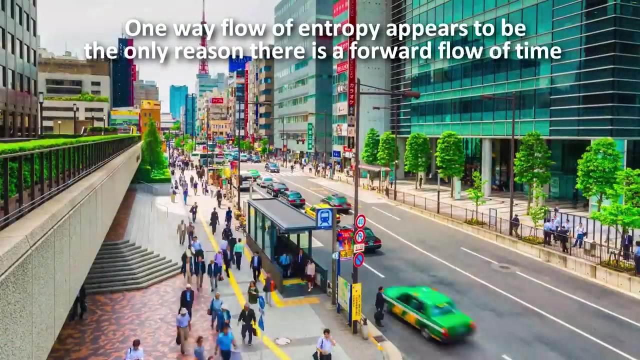 But the inside of the freezer is not an isolated system. because the refrigerator uses energy inside, It increases entropy of the room by heating up the room more than cooling what's inside the refrigerator. You should also remember this fact. The one-way flow of entropy appears to be the only reason we have a forward direction. 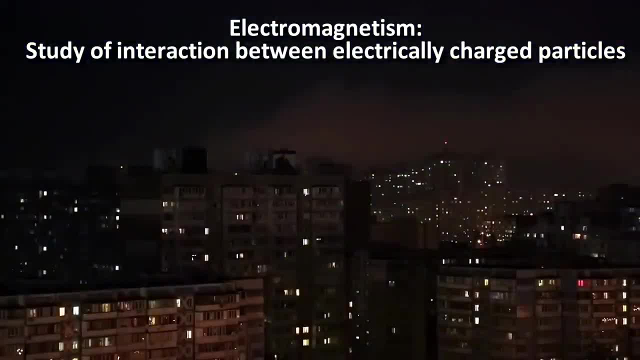 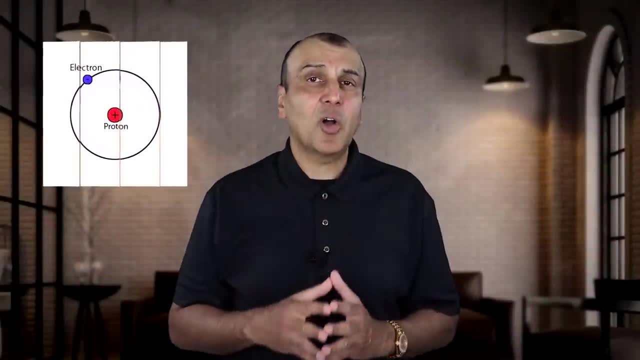 of time. Electromagnetism is the study of the interaction between electrically charged particles. The essential concepts are embodied in Maxwell's equations. Objects have something called a charge. We don't know what it is, It's just a property of certain types of matter. 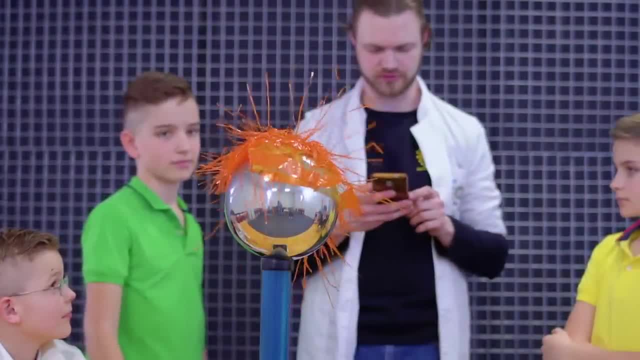 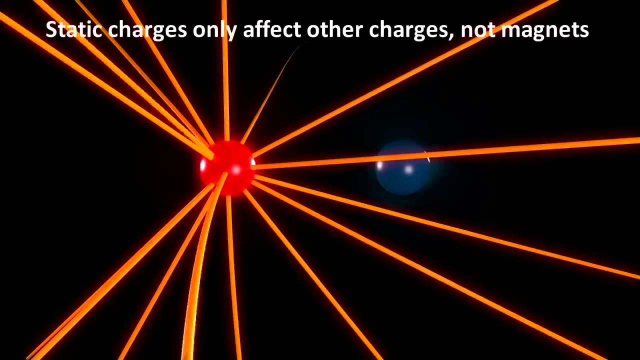 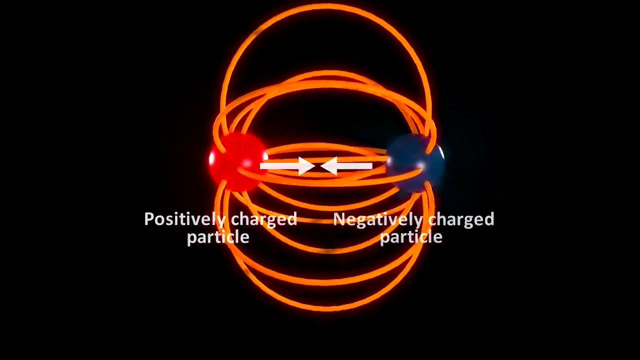 Such as electrons. If a large object has a negative charge, this means it has more electrons than protons. The first concept I want you to understand is that if you have a static object with a charge, it will affect only other charges, And if you have a static magnet, it will affect only other magnets. 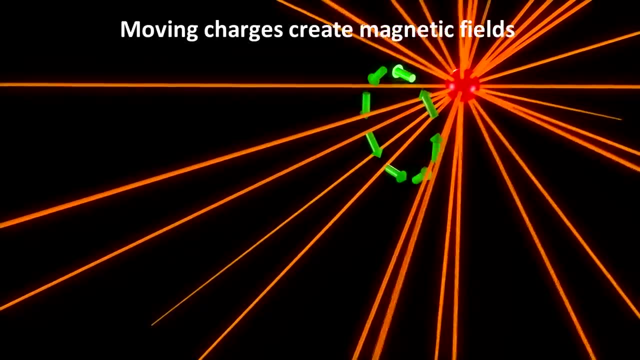 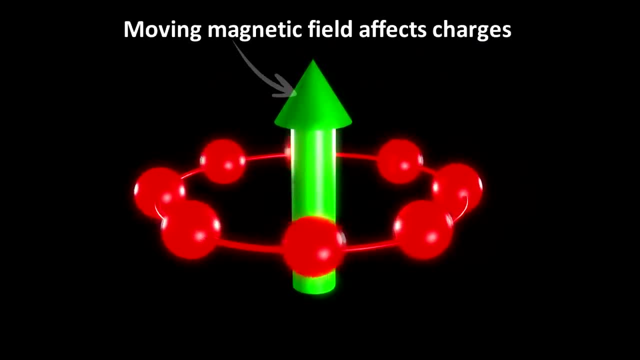 It will not affect other charges. But if you have a moving charge, it will affect a magnet, And if you have a moving magnet, it will affect a charge At the simplest level of description. That's what these four equations are all about. 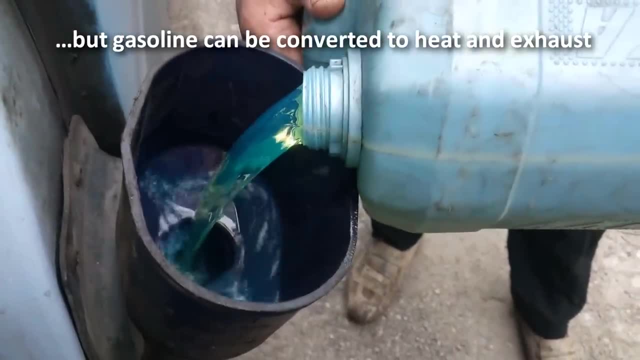 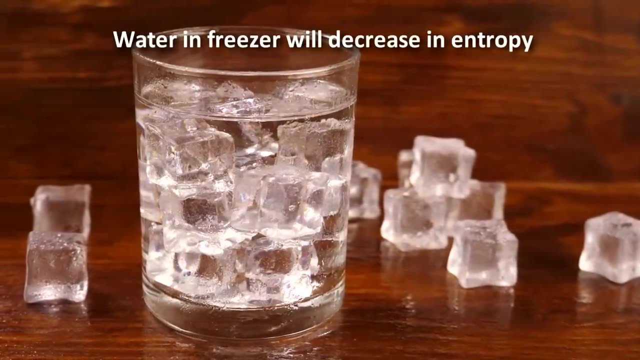 gasoline, but gasoline can be converted to heat and exhaust. It's important to remember the words isolated system. If you put a glass of water in the freezer, it will decrease the entropy, But the inside of the freezer is not an isolated system, because the refrigerator uses energy. 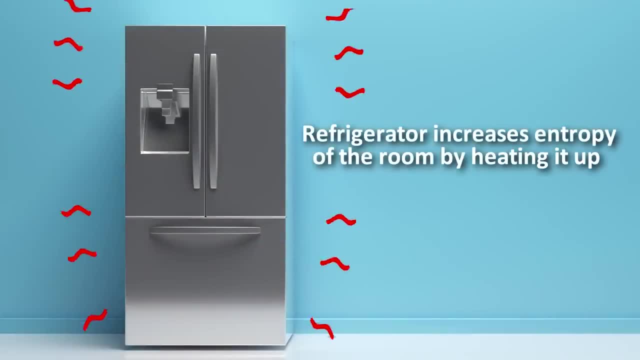 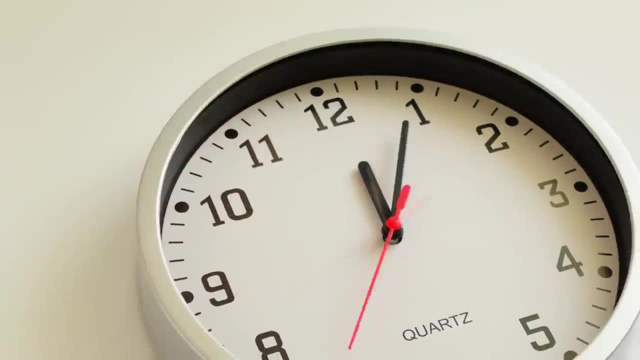 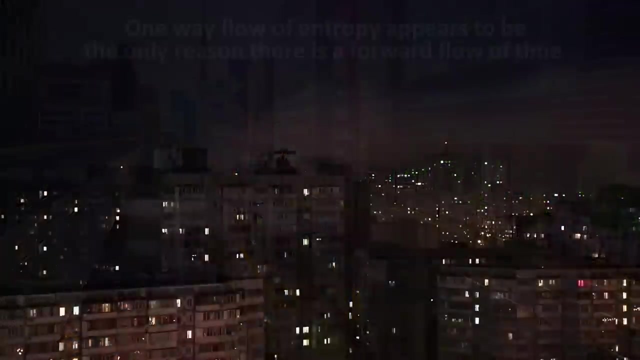 from electricity to cool the inside. It increases entropy of the room by heating up the room more than cooling what's inside the refrigerator. You should also remember this fact. The one-way flow of entropy appears to be the only reason we have a forward direction of time. Electromagnetism. 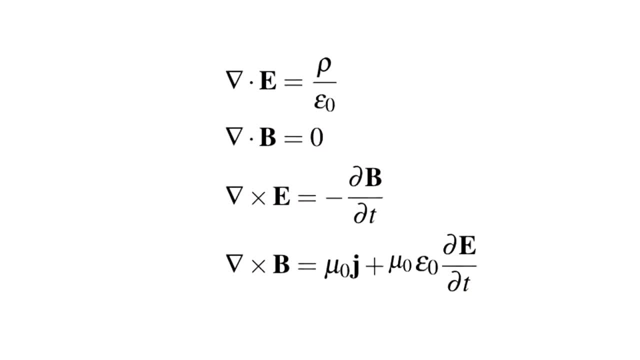 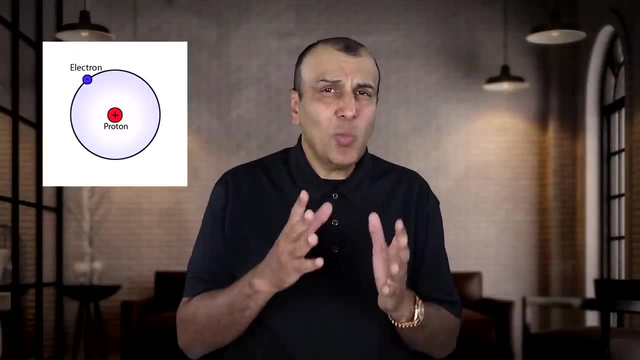 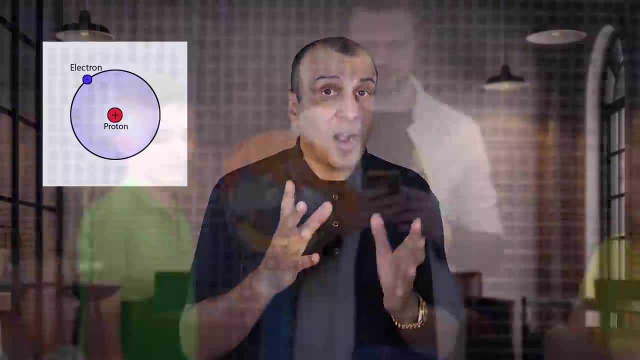 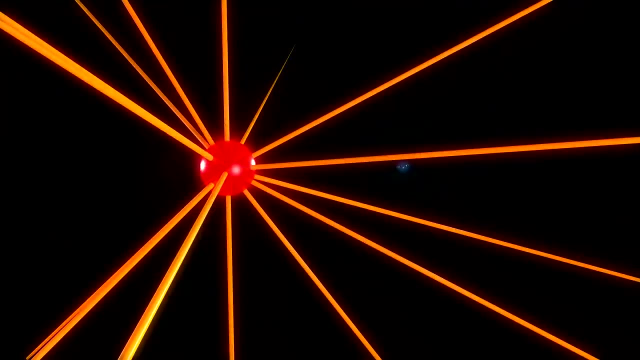 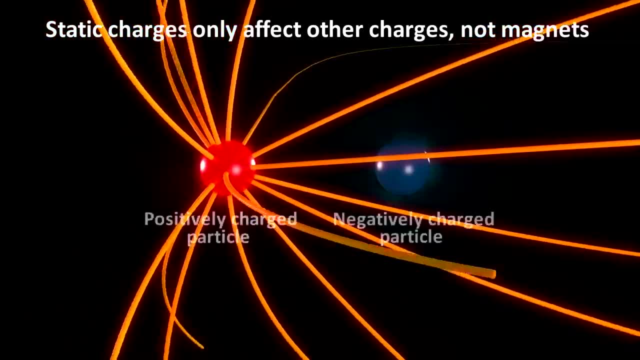 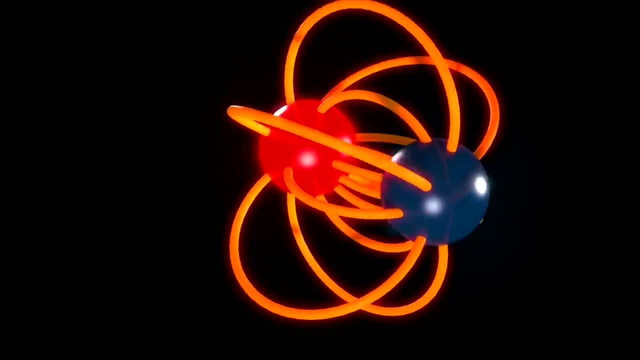 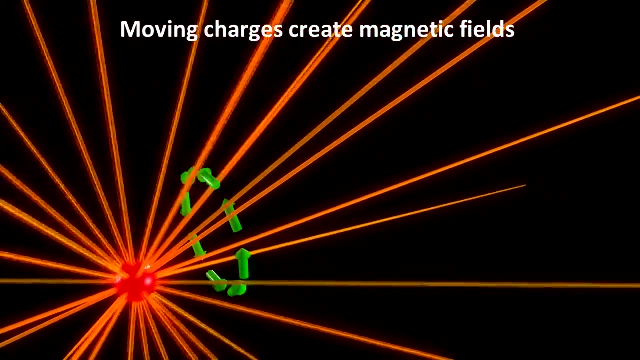 is that if you have a static object with a charge, it will affect only other charges, And if you have a static magnet, it will affect only other magnets. It will not affect other charges. But if you have a moving charge, it will affect a magnet, And if you have a moving magnet, it will affect a charge. 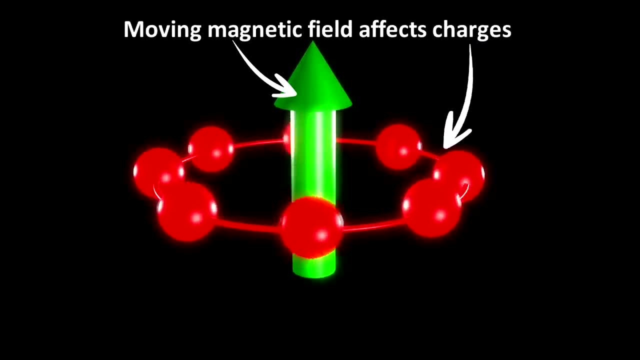 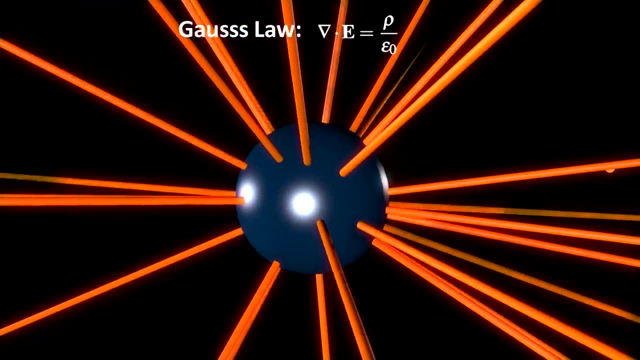 At the simplest level of description. that's what these four equations are all about. The first equation tells us that if you have an electrical charge, there will be an electrical field emanating from it. The second equation is basically the same concept for magnets, except that magnets 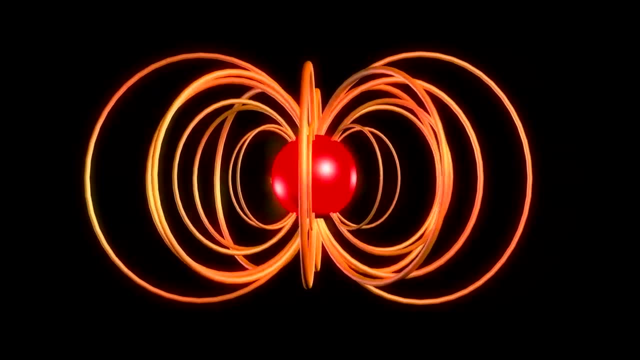 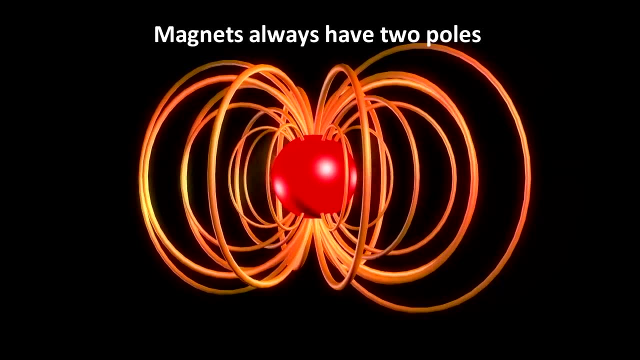 will always have as many field lines going out as coming back in. Another way to say this is that magnets will always have two poles: a positive and a negative pole. It can never be a monopole. You can keep breaking up the magnet, but it will always fall. 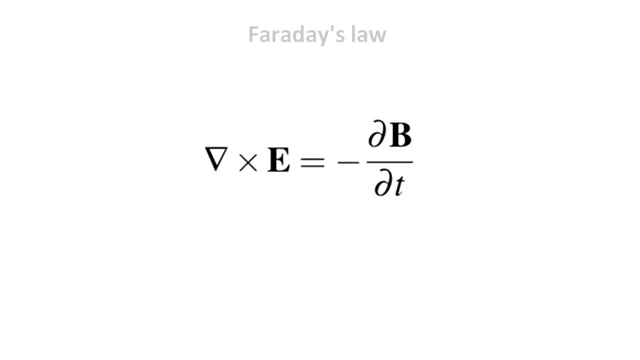 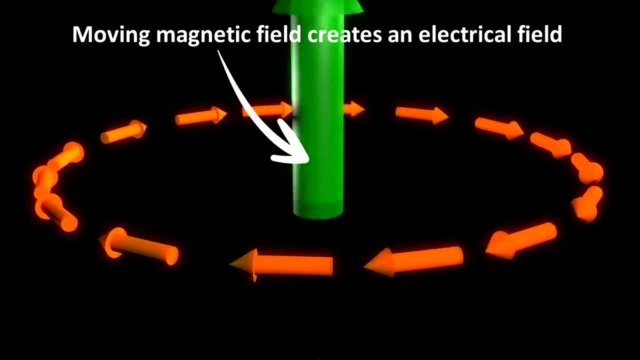 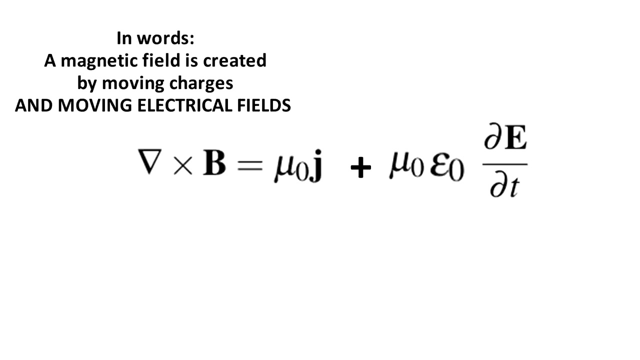 The third equation says that if you move a magnet, you will create an electrical field. This means that if a charge is nearby, it will feel a force. This is how electricity is generated: by moving magnets. The fourth equation says that a moving charge or moving electrical field creates a 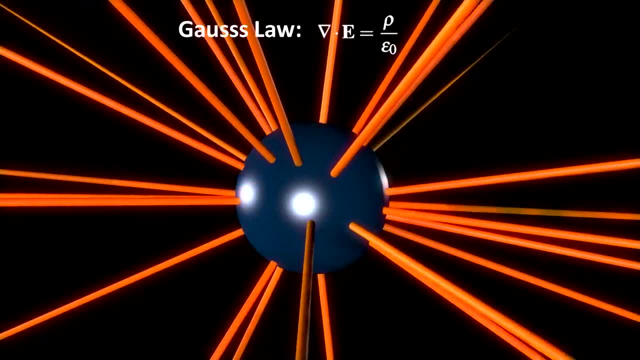 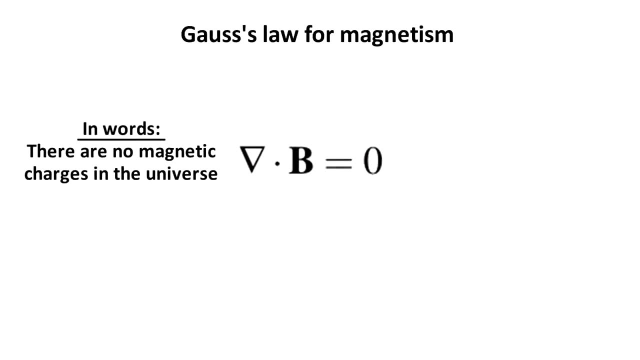 The first equation tells us that if you have an electrical charge, there will be an electrical field emanating from it. The second equation is basically the same concept for magnets, except that magnets will always have as many field lines going out as coming back in. 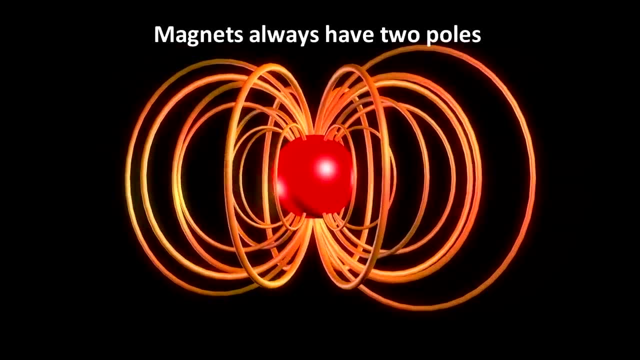 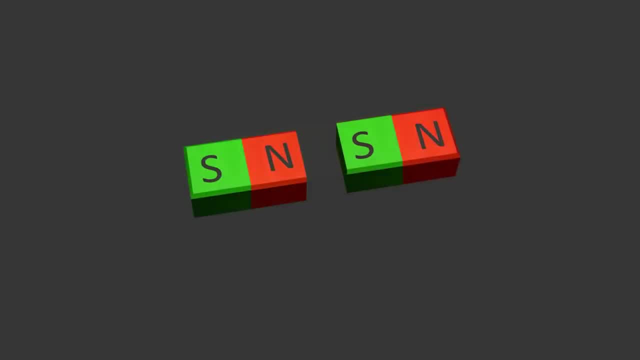 Another way to say this is that magnets will always have two poles, A positive and a negative pole. It can never be a monopole. You can keep breaking up the magnet, but it will always form a new magnet with two poles. The third equation says that if you move a magnet, you will create an electrical field. 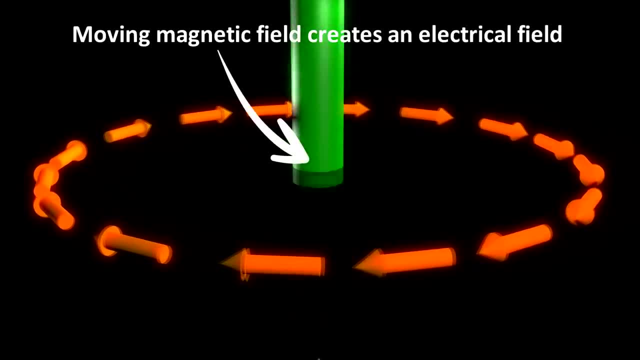 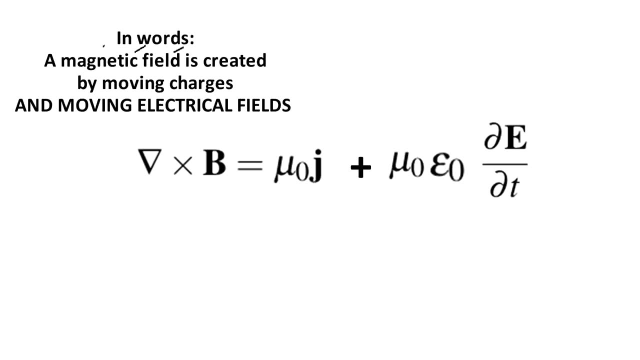 This means that if a charge is nearby, it will feel a force. This is how electricity is generated: by moving magnets. The fourth equation says that a moving charge or moving electrical field creates a magnetic field. I want you to take note of two constants, mu-naught and epsilon-naught, which are the 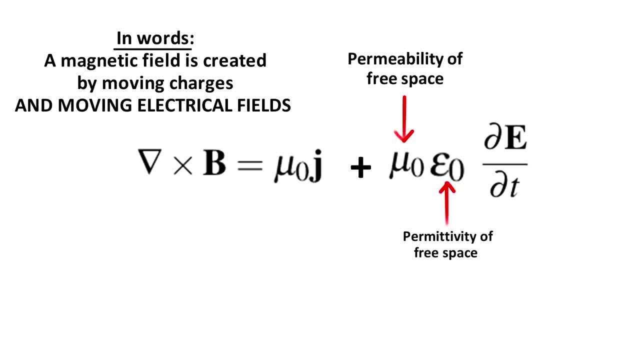 permeability and permittivity of free space respectively. These two constants determined the speed of light, because these two constants measure the distance of space to changing electrical and magnetic fields. This brings us to Albert Einstein and his theory of relativity, who ushered in a revolution. 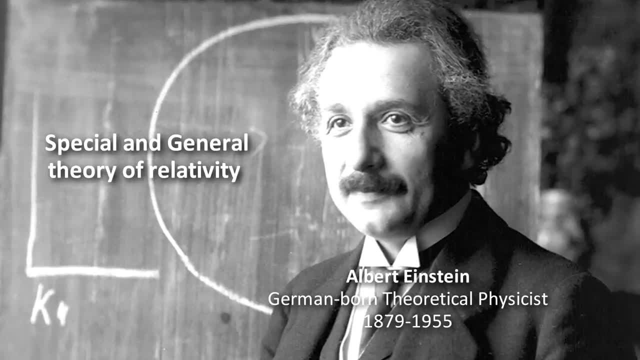 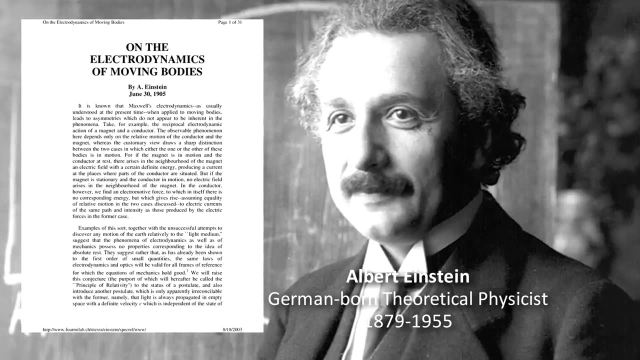 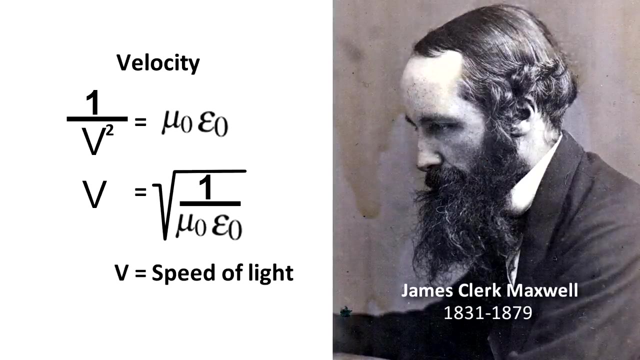 in physics. Interestingly, the title of his 1905 paper on special relativity was called On the Electrodynamics of Moving Bodies. This tells you how tied this theory is to Maxwell's ideas. Einstein thought that if the speed of light was determined by two constants, 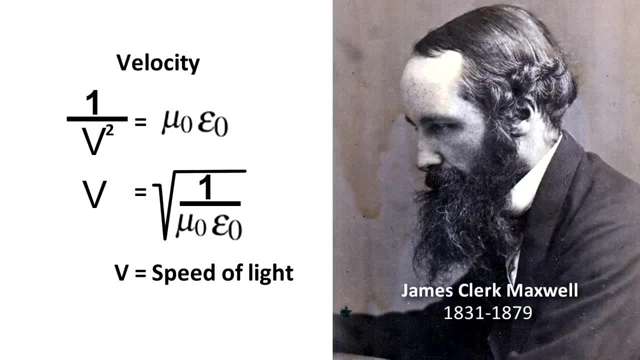 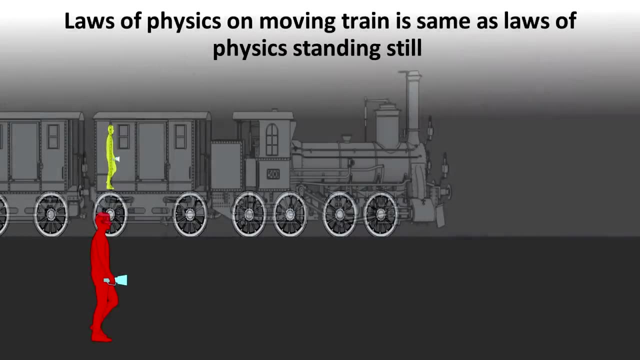 mu naught and epsilon naught then. the speed of light is a constant too, and may not change in any frame of reference. This was one of the postulates of special relativity. The second postulate was the principle of relativity, meaning the laws of physics are the same for. 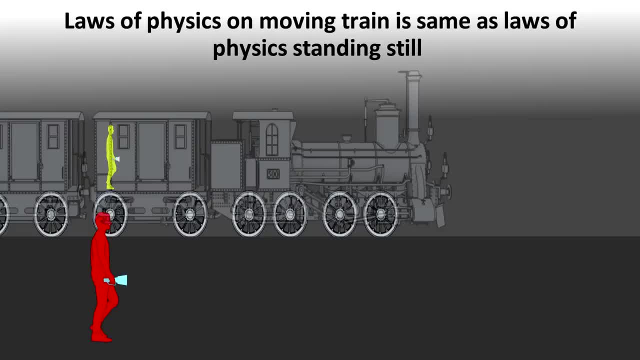 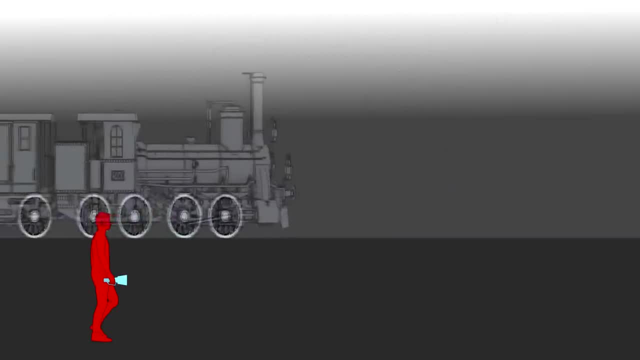 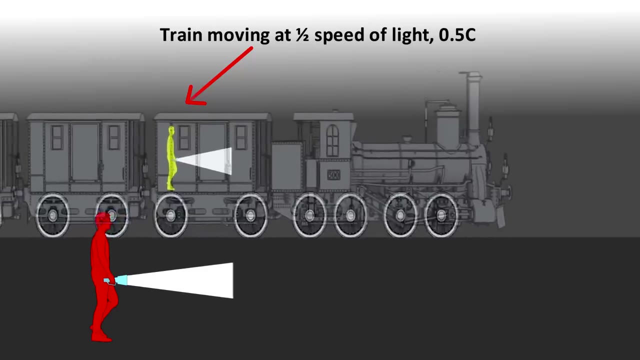 all observers who are moving at the same velocity relative to each other. If these two assumptions were correct, this had some major implications. Suppose you are stationary next to a train moving at half the speed of light And you turn on a flashlight in the direction of the moving train. Suppose another person- 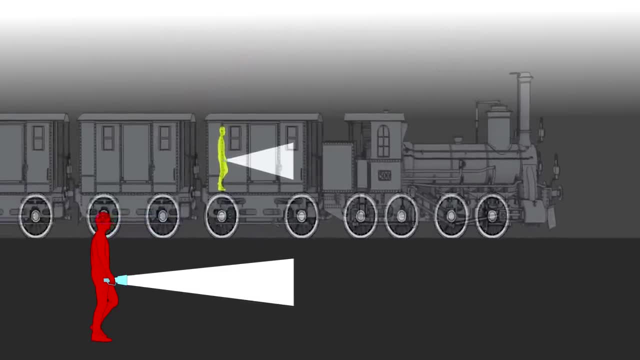 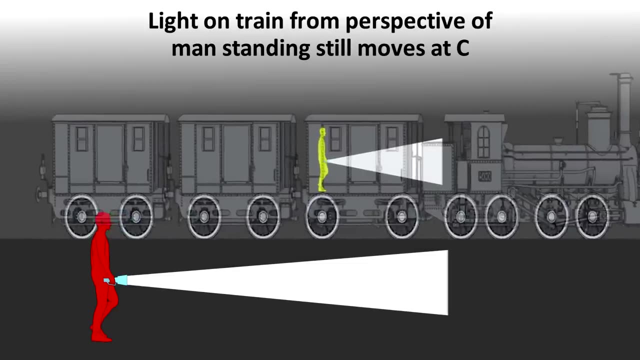 is on the train and turns on an identical flashlight at exactly the same moment. If you saw the light beam on the train, you might think that it should be moving at one and a half times the speed of light, But it doesn't. It moves at exactly one times the speed of. 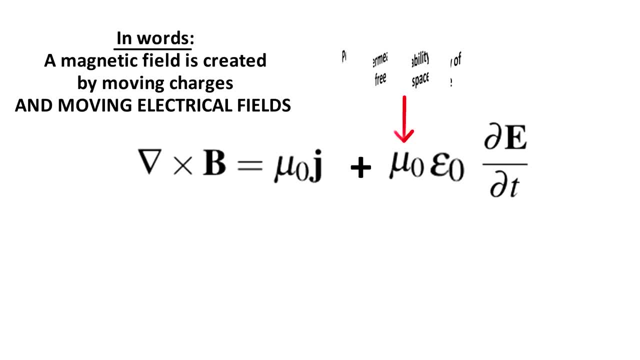 magnetic field. I want you to take note of the constants mu naught and epsilon naught, which are the permeability and permittivity of free space respectively. These two constants determine the speed of light because they measure the resistance of space to changing electrical and magnetic 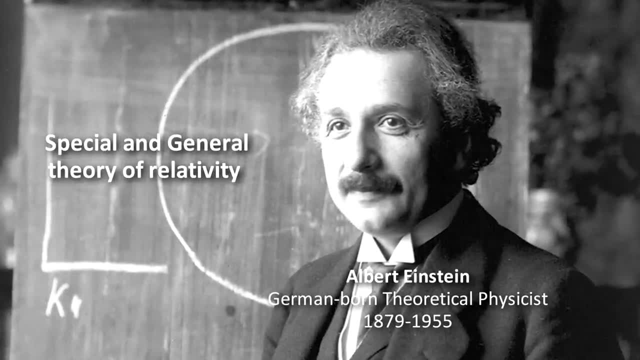 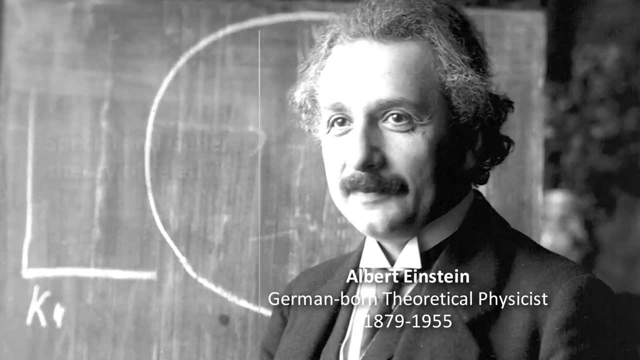 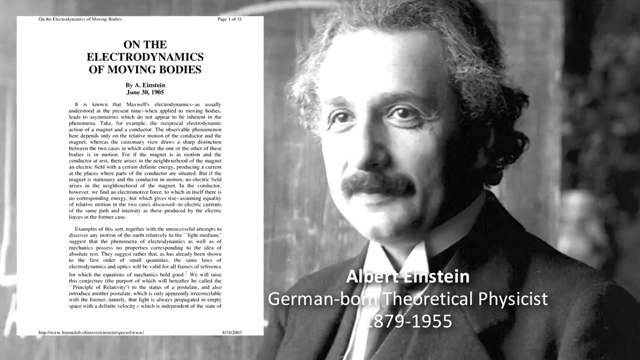 fields. This brings us to Albert Einstein and his theory of relativity, who ushered in a revolution in physics. Interestingly, the title of his 1905 paper on special relativity was called On the Electrodynamics of Moving Bodies. This tells you how tied this theory is to Maxwell's. 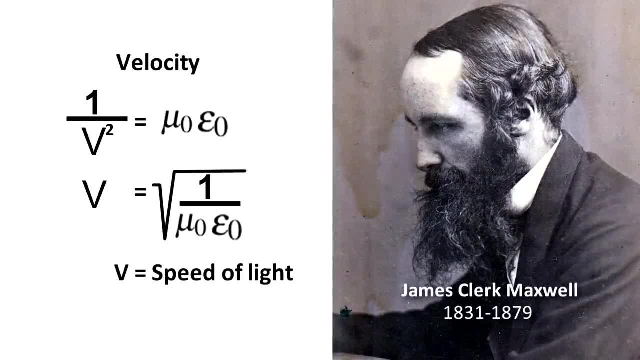 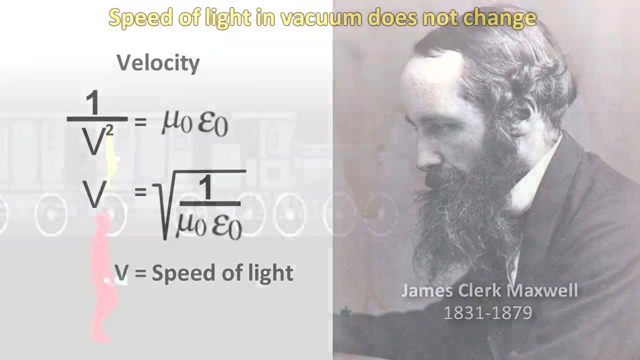 ideas. Einstein thought that if the speed of light was determined by two constants- mu naught and epsilon naught- then the speed of light is a constant too, and may not change in any frame of reference. This was one of the postulates of special relativity. The second: 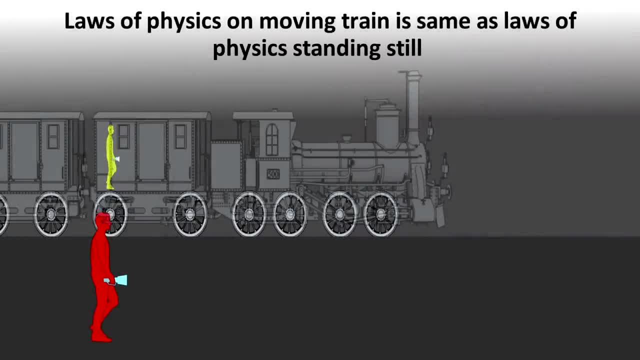 postulate was the principle of relativity, meaning the laws of physics are the same for all observers who are moving at the same velocity relative to each other. If these two assumptions were correct, this had some major implications. Suppose you're stationary next to a train moving at half the 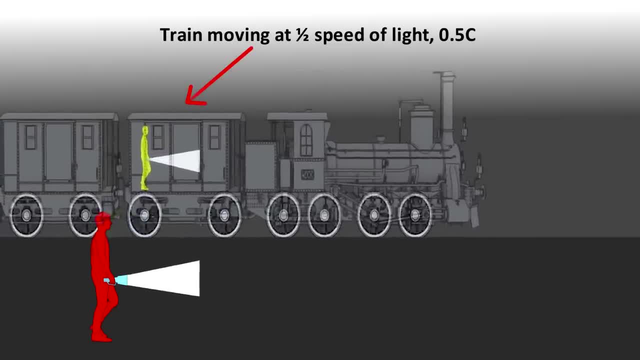 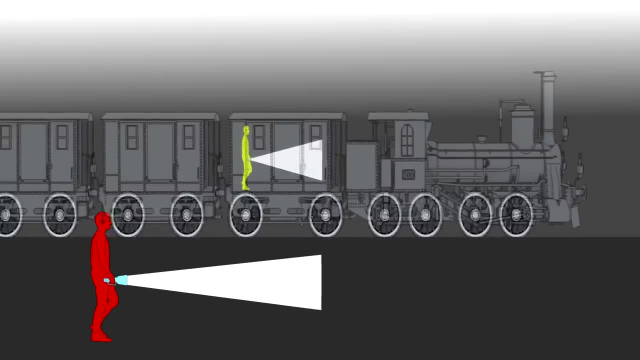 speed of light and you turn on a flashlight in the direction of the moving train. Suppose another person is on the train and turns on an identical flashlight at exactly the same moment. If you saw the light beam on the train, you might think that it should be moving at one and a half times the 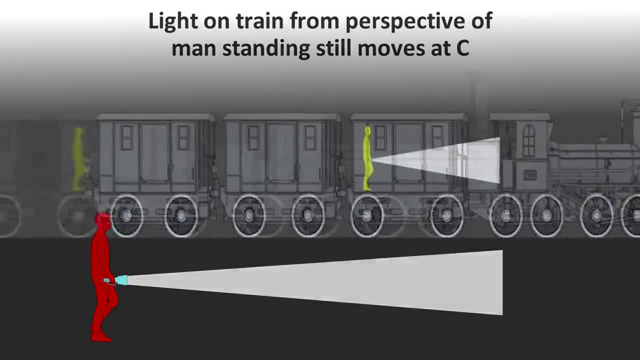 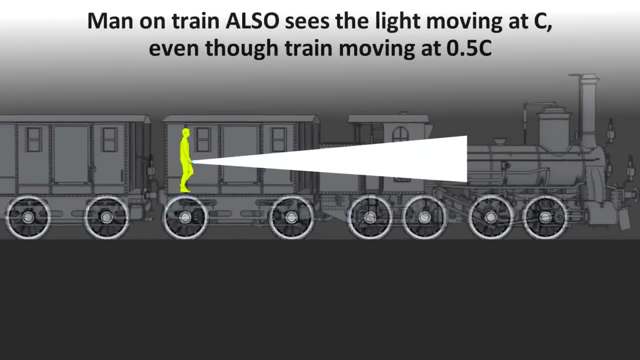 speed of light. but it doesn't. It moves at exactly one times the speed of light. Does this mean that the man on the train sees the speed of light moving at half the speed of light? No, because of the principle of relativity. 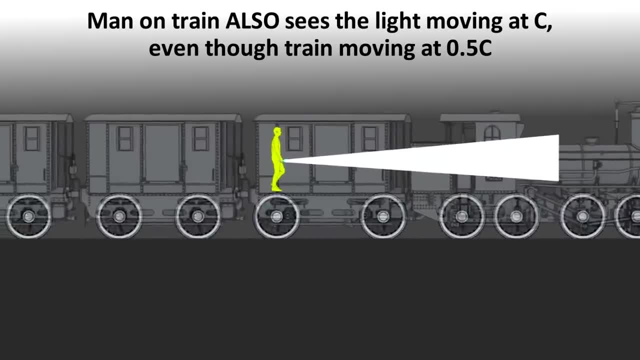 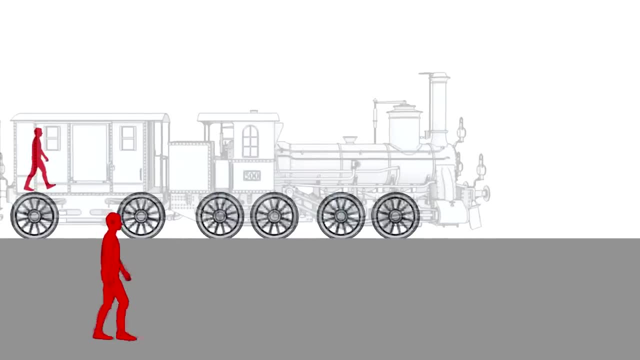 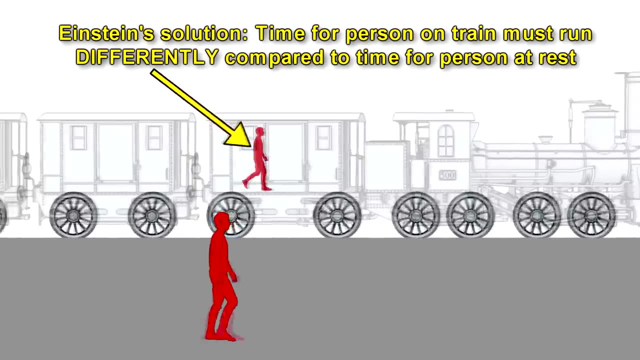 from his flashlight, traveling at exactly one times the speed of light c. This appears to be a paradox. How can these two observations be reconciled? What Einstein showed is that the only way this can happen is if time for the person on the train slows down. from the perspective of 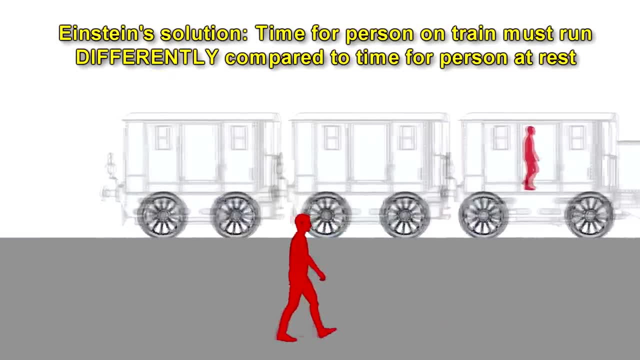 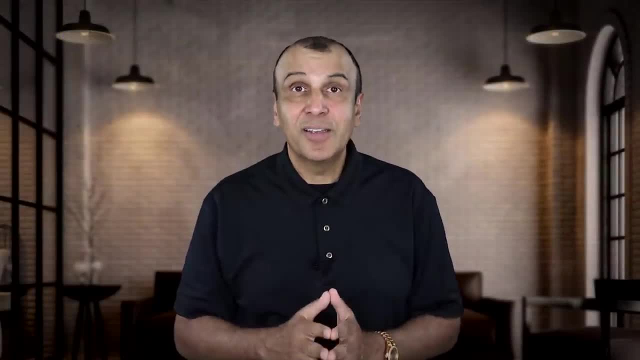 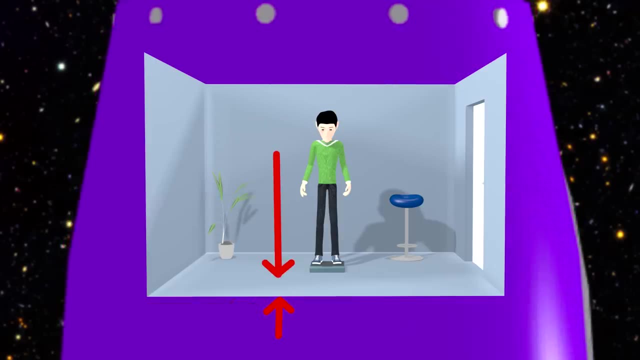 someone standing still. This was the crucial, paradigm shifting insight that he unleashed on humanity: Time was not fixed, It was relative. Later, Einstein, with his theory of general relativity, showed that, using the same general assumptions, there would be no way to tell. if you 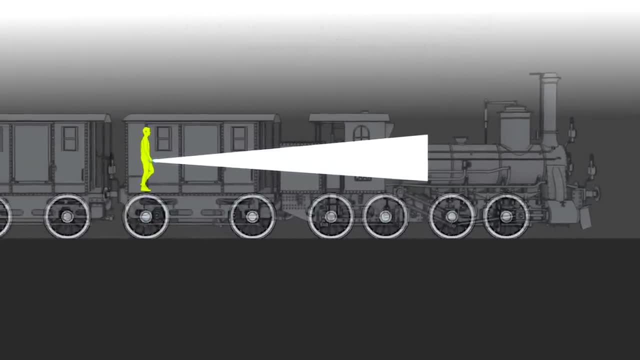 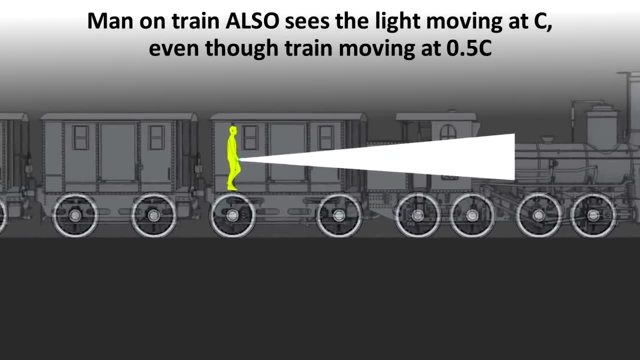 light. Does this mean that the man on the train sees the speed of light moving at half the speed of light? No, because of the principle of relativity, He also sees the beam of light moving at half the speed of light from his flashlight, traveling at exactly one times. 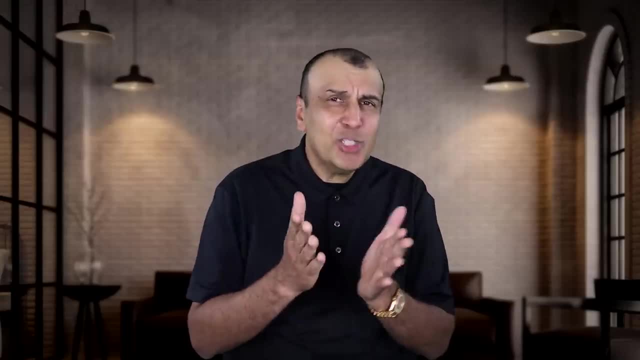 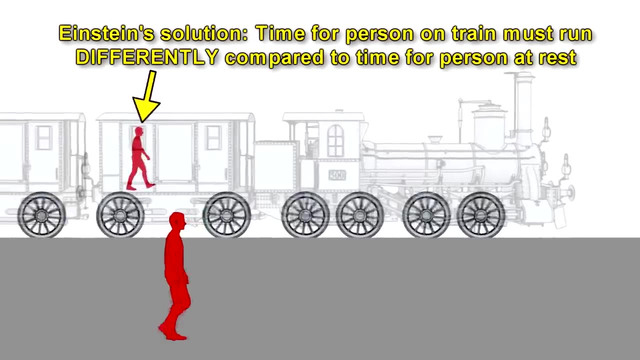 the speed of light c. This appears to be a paradox. How can these two observations be reconciled? What Einstein showed is that the only way this can happen is if time for the person on the train slows down from the perspective of someone standing still. This: 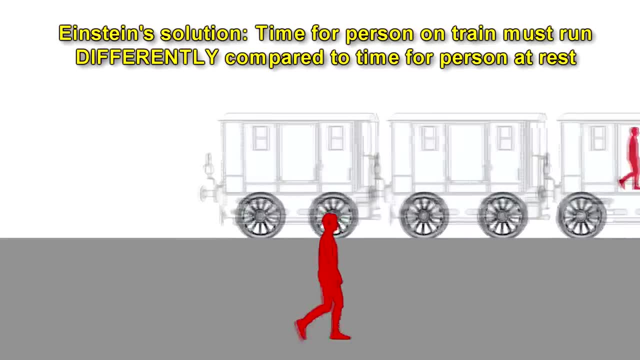 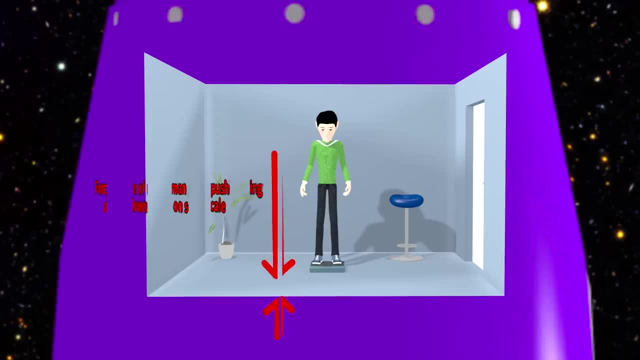 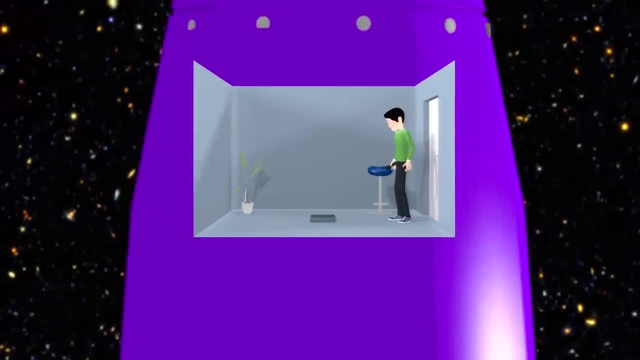 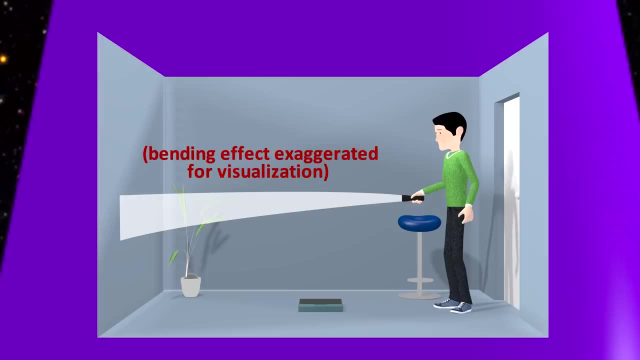 or standing stationary on earth. So, for example, if you were on a spaceship moving at the same acceleration as gravity- 9.8 meters per second squared- and you held a flashlight perpendicular to the direction of acceleration, the light would appear to bend because the wall would 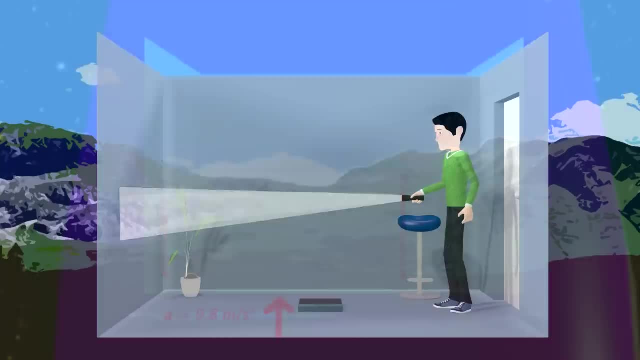 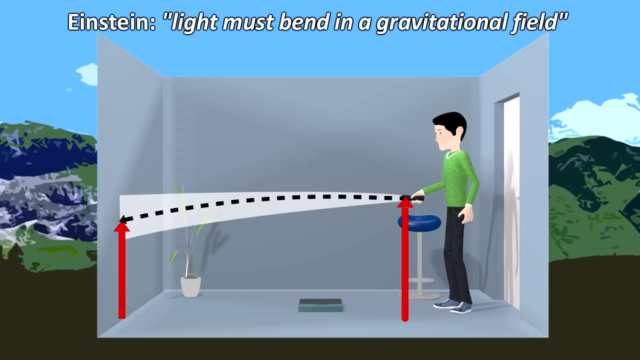 be rushing upward at ever faster speeds. This means that if you were anywhere on earth standing still and you did the same experiment, your light beam would appear to bend, because the acceleration due to gravity is 9.8 meters per second squared. But since light always takes, 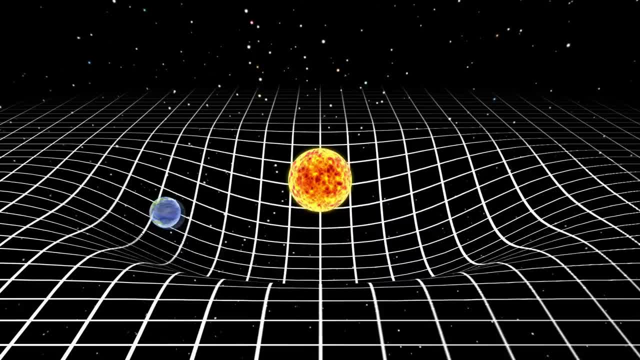 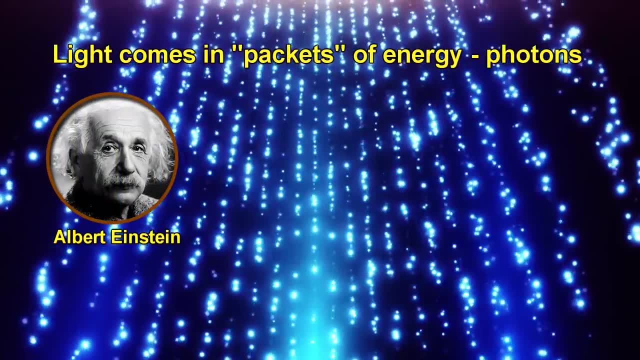 the shortest path between any two points. this means that space-time itself must be bending in order for light to take that path. The bent path is the shortest path, just like the shortest paths on the surface of the earth are bent. I find it ironic that Einstein, although he was one of the founders of quantum mechanics, 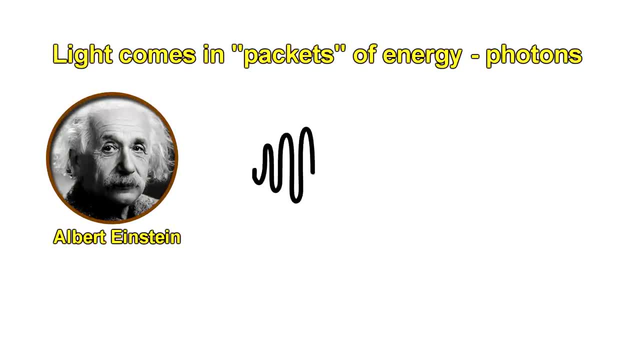 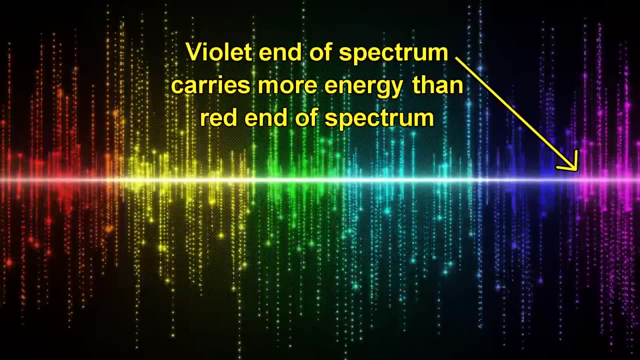 because he showed that light came in packets of energy called quanta. we now call them photons. yet he largely stayed resistant to the main implications of quantum mechanics, and that is the idea of a probabilistic and non-deterministic nature of quantum particles. 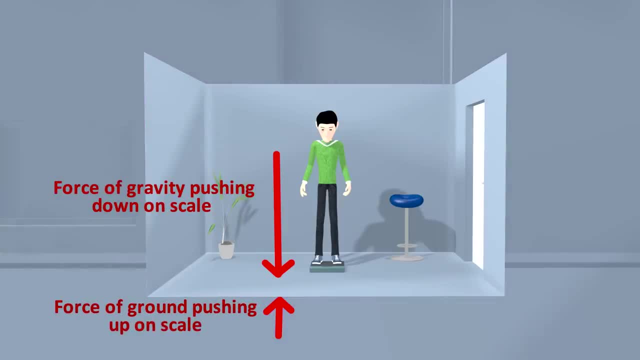 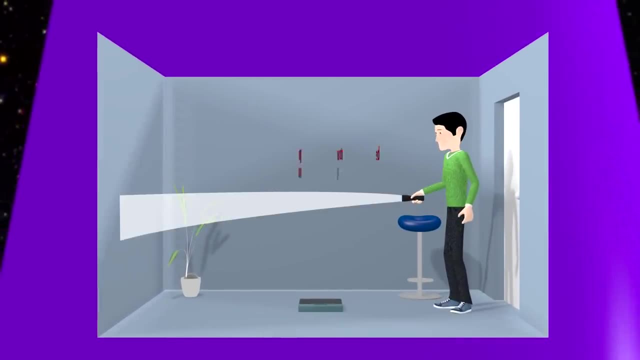 were on an accelerating reference frame or standing stationary on earth. So, for example, if you were on a spaceship moving at the same acceleration as gravity- 9.8 meters per second squared- and you held a flashlight perpendicular to the direction of acceleration, the light would appear to bend. 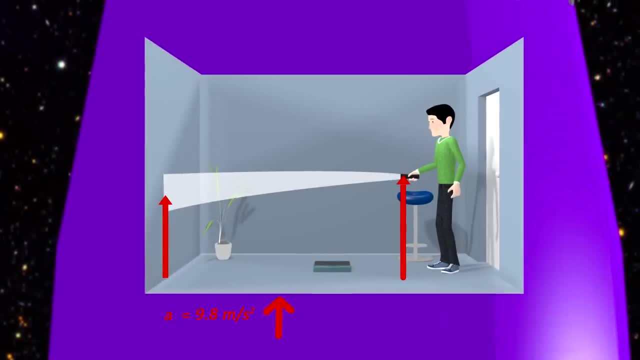 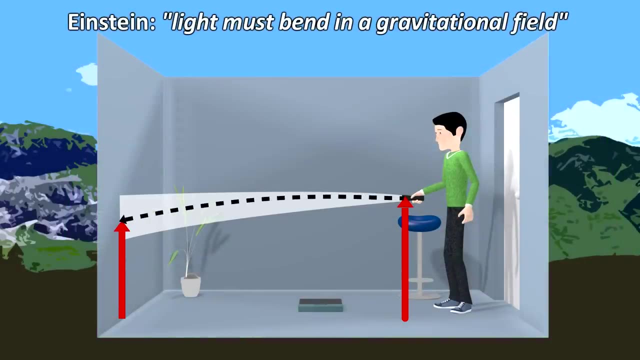 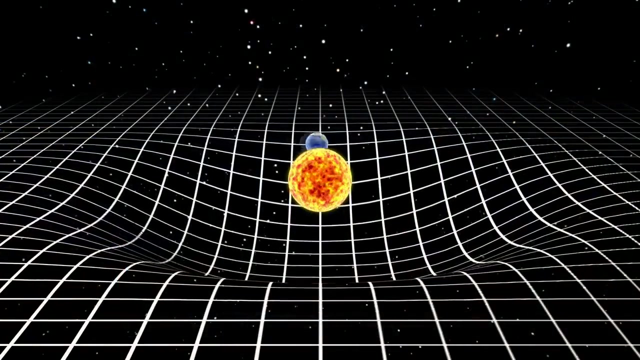 because the wall would be rushing upward. This means that if you were anywhere on earth standing still and you did the same experiment, your light beam would appear to bend, because the acceleration due to gravity is 9.8 meters per second squared. But since light always takes the shortest path between any two points, this means 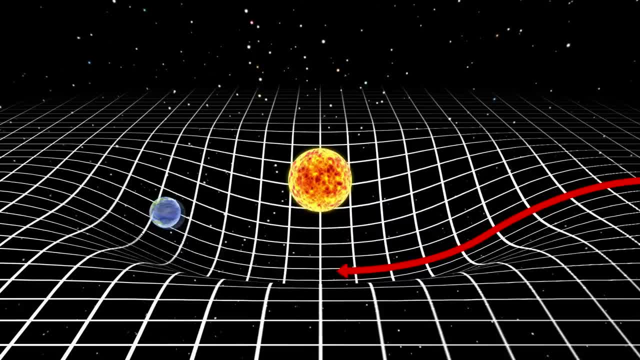 that space-time itself must be bending in order for light to take that path. The bent path is the shortest path, just like the shortest paths on the surface of the earth are bent. I find it ironic that Einstein's theory of general relativity is completely different from the theory of gravity. 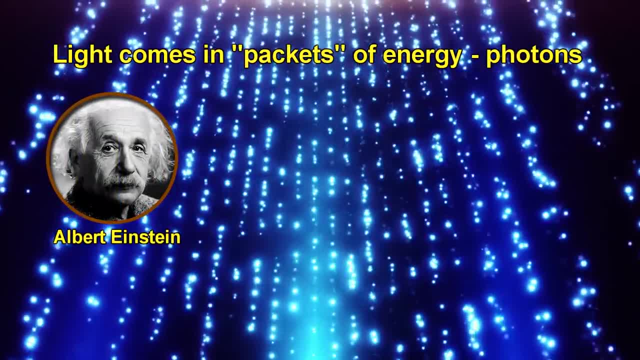 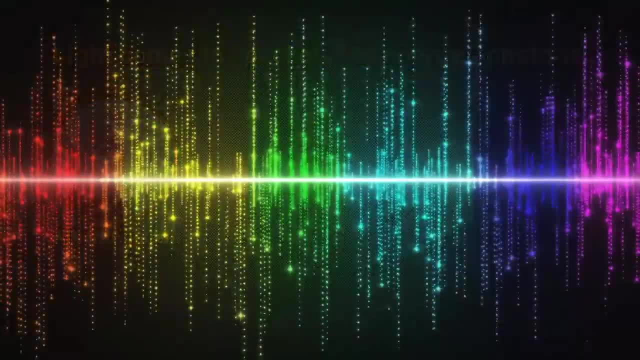 Although he was one of the founders of quantum mechanics, because he showed that light came in packets of energy called quanta- we now call them photons- Yet he largely stayed resistant to the main implications of quantum mechanics, and that is the idea of a probabilistic and non-deterministic 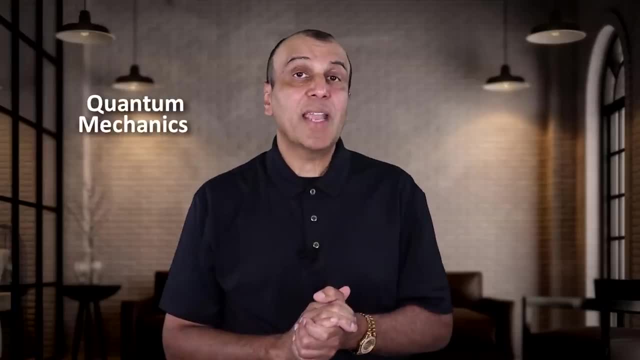 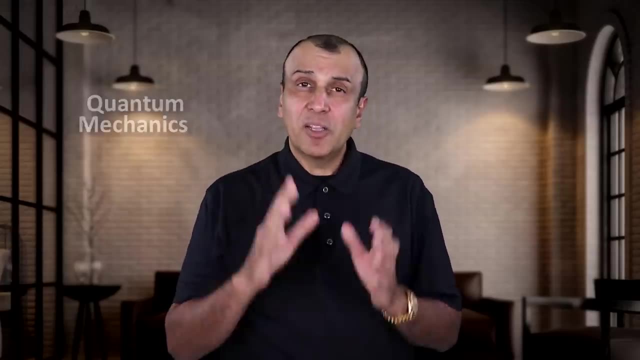 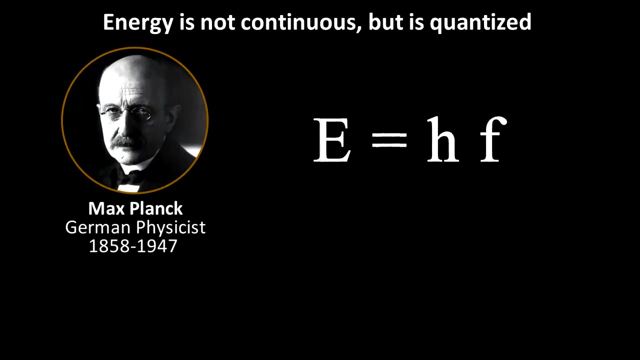 nature of quantum particles. There are many equations of quantum mechanics, but in my view there are three principles that are the most important to remember, and they are expressed in three equations. The first equation was championed by Max Planck. Our first equation is called Planck's constant, which is arguably the father of quantum mechanics. It 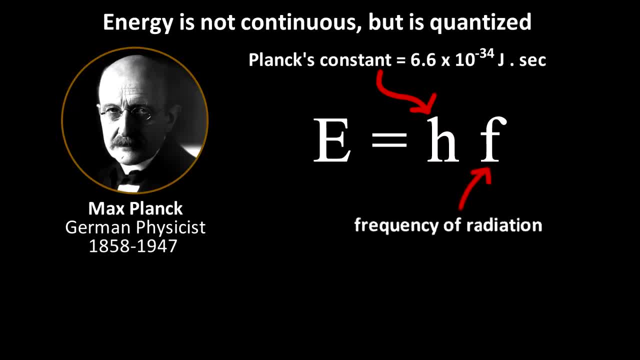 says that energy is not continuous, but it is quantized. The energy absorbed or emitted by materials can only occur in distinct quanta of energy, and the amount of energy equals the frequency of the radiation times, a constant called Planck's constant. Using this concept, 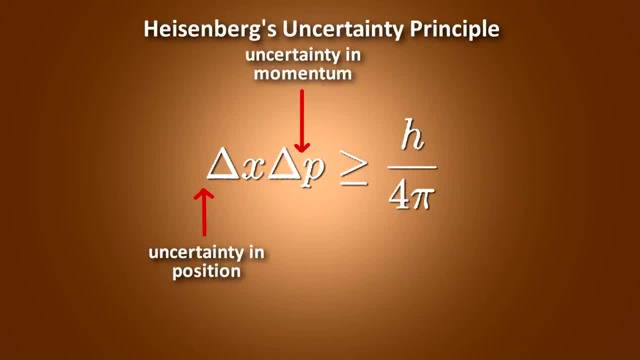 Einstein later showed that a photon is both a wave and a particle. The second idea is expressed by the Heisenberg uncertainty principle: know both a particle's exact position and its exact momentum at the same time. For a particle with mass, this means that if you know exactly where a particle is, you don't. 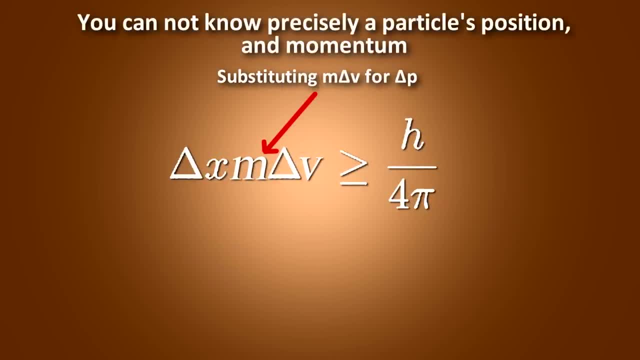 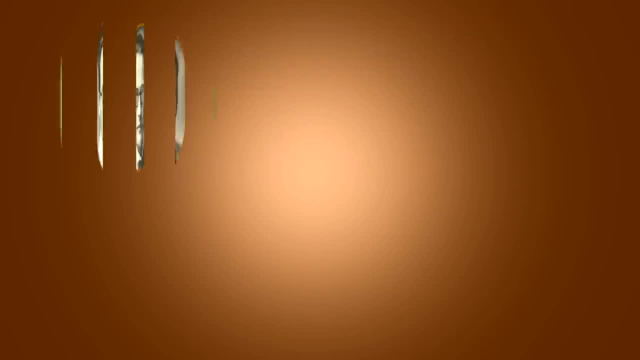 know how fast it's going. And if you know exactly how fast it's going, you have no idea where the heck it is. There is an inherent uncertainty associated with quantum particles. The third equation comes from Schrodinger's equation. It basically says that prior to 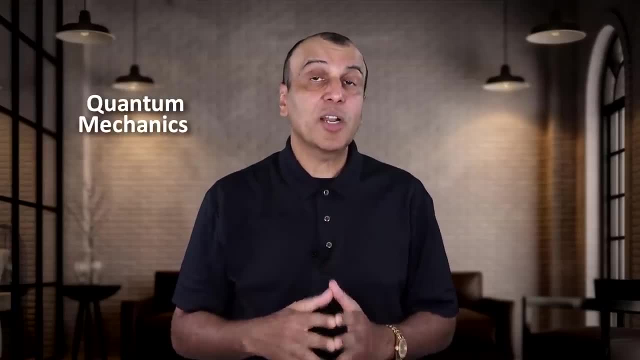 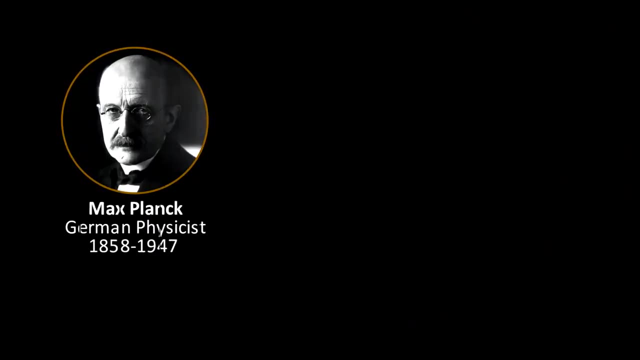 There are many equations in quantum mechanics, but in my view, there are three principles that are the most important to remember, And they are expressed in three equations. The first equation was championed by Max Planck, arguably the father of quantum mechanics. 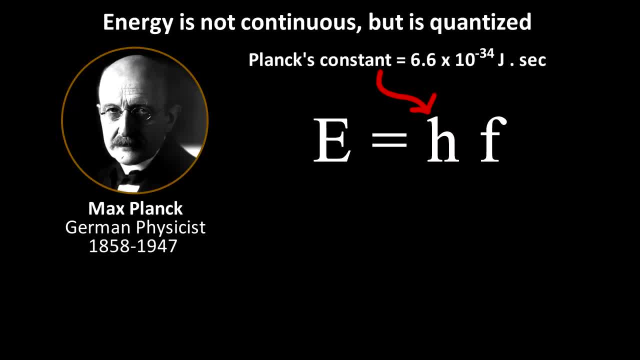 It says that energy is not continuous, but it is quantized. The energy absorbed or emitted by materials can only occur in distinct quanta of energy, and the amount of energy equals the frequency of the radiation times, a constant called Planck's constant. Using this concept, 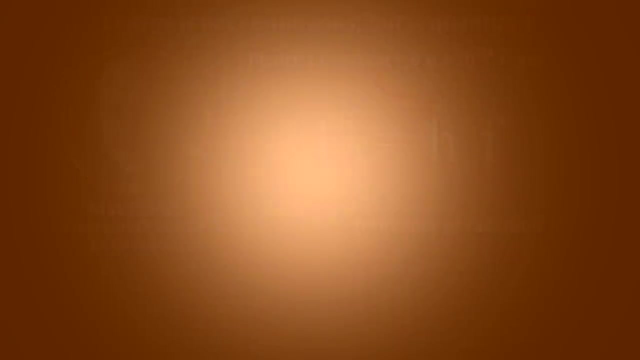 Einstein later showed that a photon is both a wave and a particle. The second idea is expressed by the Heisenberg uncertainty principle. It basically says that you cannot know both a particle's exact position and its exact momentum. This means that the mass of a particle means that if you know exactly where a particle is, you don't know. 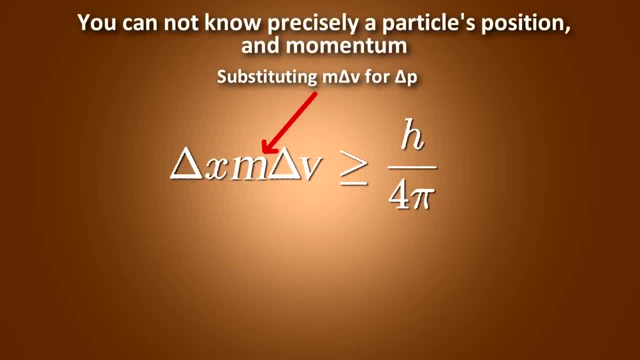 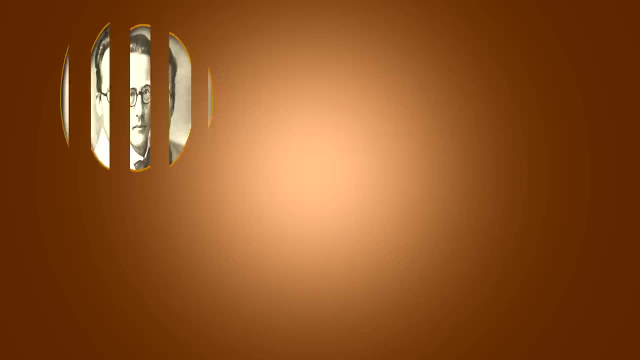 how fast it is going. And if you know exactly how fast it is going, you have no idea where the heck it is. There is an inherent uncertainty associated with quantum particles. The third equation comes from Schrodinger's equation. It basically says that prior to 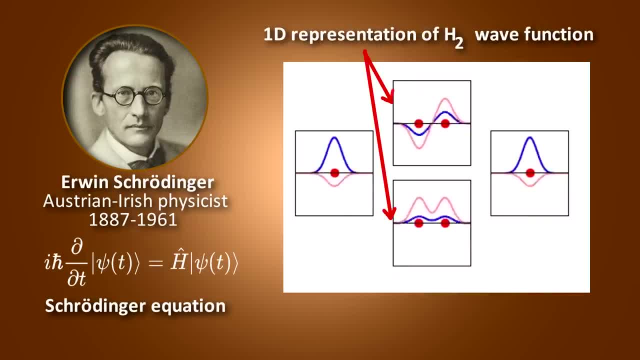 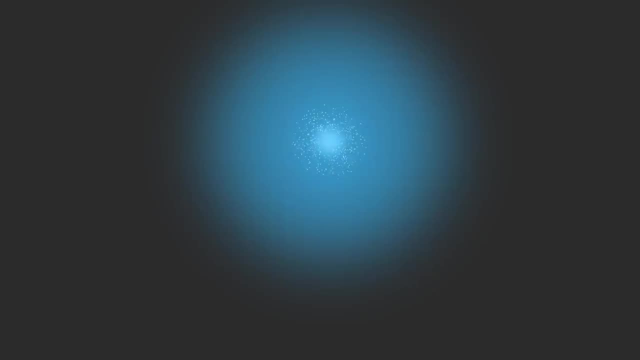 measurement quantum systems are in superposed states. This means that their properties can only be expressed in terms of a wave function. A wave function, crudely simplified, is a set of probabilities. So, for example, in a hydrogen atom, you can't know where to find the electron in advance. All you can know. 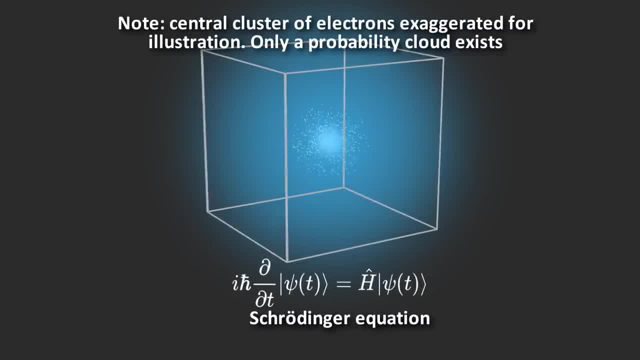 is the probability of where you might find it if you measured it Prior to measurement. all quantum systems are three-dimensional clouds or waves of probabilities. The electron is everywhere at once. It's not here or there. It's here and there. This is not a limitation. 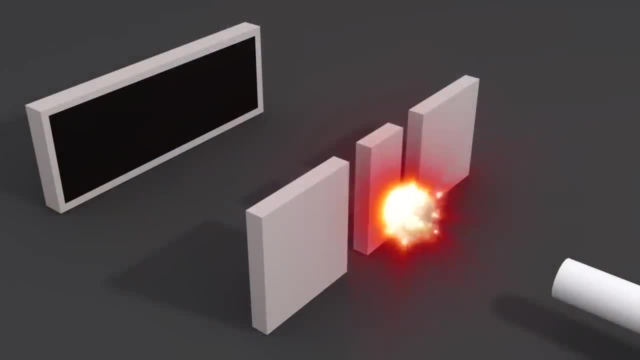 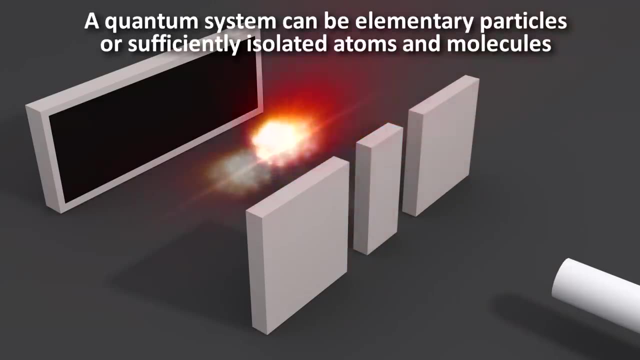 of our measuring devices. It is a limitation of reality, And this is the reason. quantum systems are so complex that they are so complex that they behave so mysteriously in the double-slit experiment. A quantum system can be an elementary particle like an electron, or even atoms and molecules. 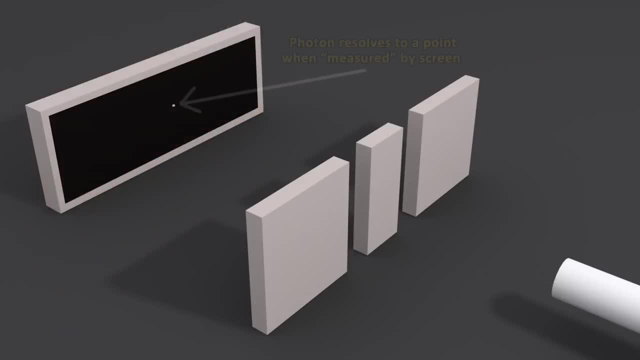 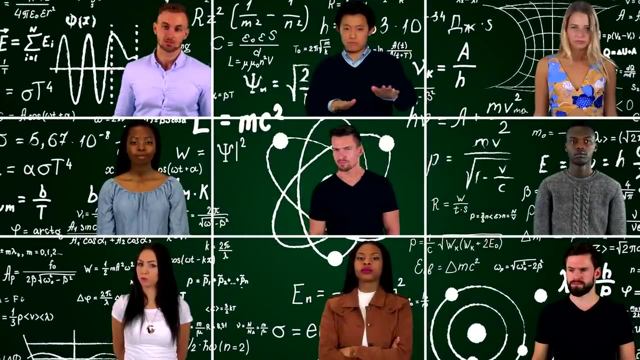 that are sufficiently isolated. Isolated means that they haven't interacted with something that would cause their wave function to collapse. This is the non-deterministic reality that Einstein had a hard time accepting and indeed, many people today still have a hard time accepting. 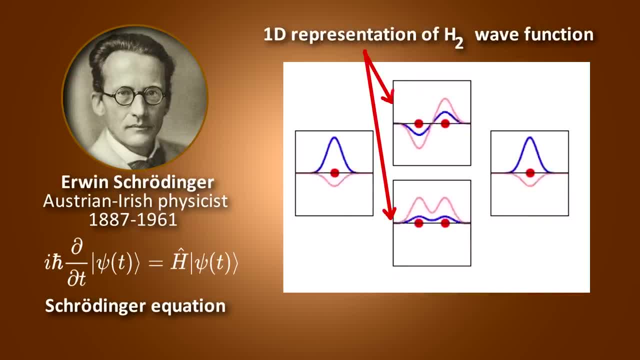 measurement quantum systems are in superposed states. This means that their properties can only be expressed in terms of a wave function. A wave function, crudely simplified, is a set of probabilities. So, for example, in a hydrogen atom, you can't know where to. 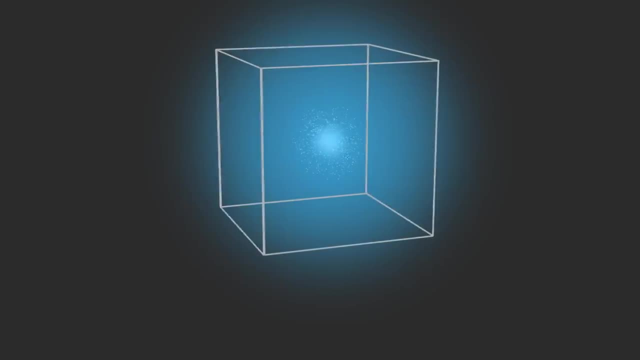 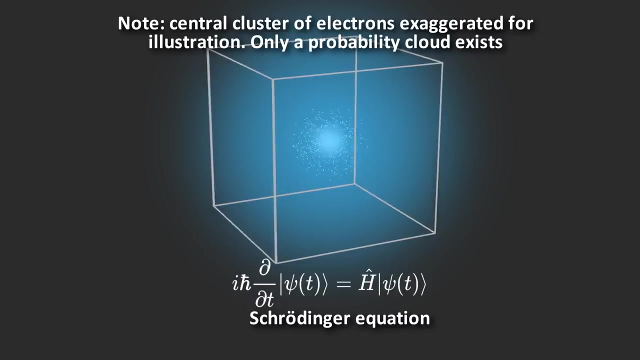 find the electron in advance. All you can know is the probability of where you might find it if you measured it Prior to measurement. all quantum systems are three-dimensional clouds or waves of probabilities. The electron is everywhere at once. It's not here, or 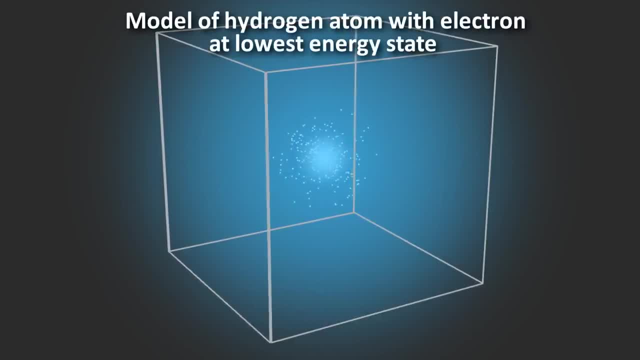 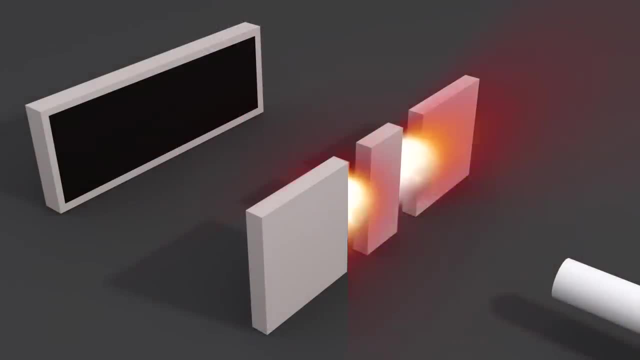 there. It's here and there. This is not a limitation of our measuring devices. It is a limitation of reality, And this is the reason quantum systems behave so mysteriously. in the double-slit experiment, A quantum system can be an elementary particle like an electron. 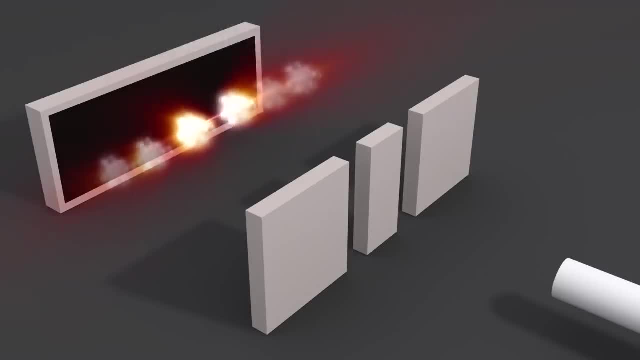 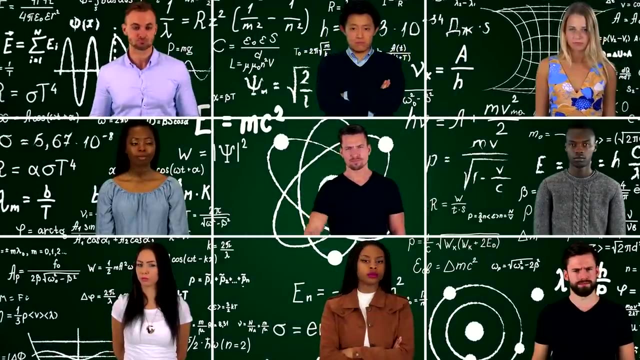 or even atoms and molecules that are sufficiently isolated. Isolated means that they haven't interacted with something that would cause their wave function to collapse. This is the non-deterministic reality that Einstein had a hard time accepting, And indeed many people. 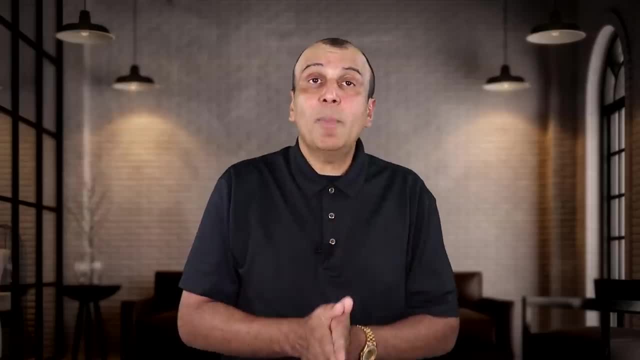 today still have a hard time accepting. But the universe has no obligation to make sure we feel comfortable about the true nature of the universe. The universe has no obligation to make sure we feel comfortable about the true nature of the universe. The universe has no obligation to make sure we feel comfortable about the true nature of reality. 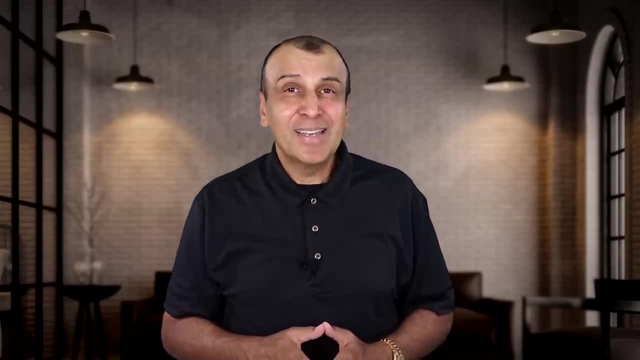 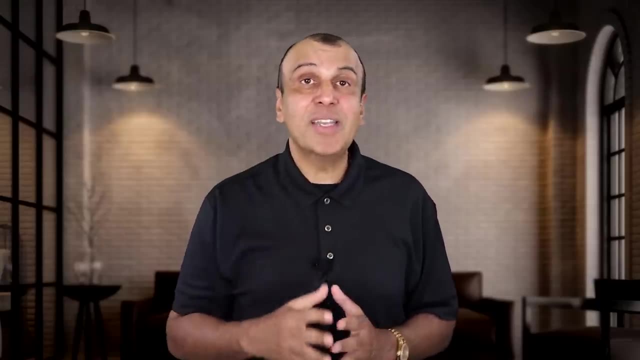 Now, this is just one bald ape's opinion about what he thinks are the most important concepts in physics worth remembering, so I hope you found it useful. Now, if you'd like to learn these subjects more in-depth, then you're not going to find a better on-demand. 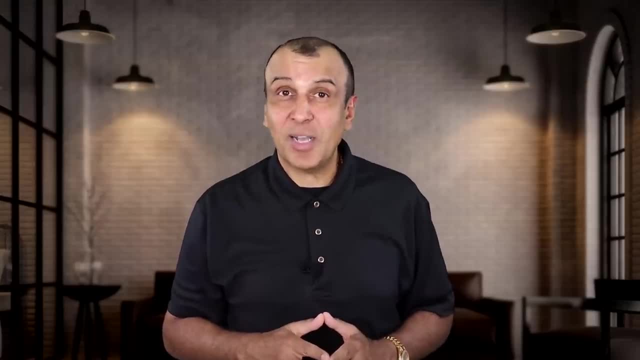 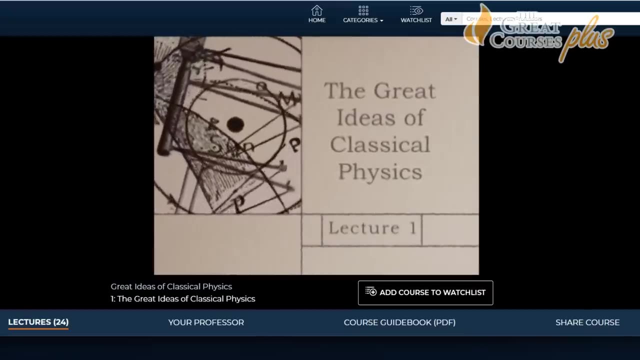 video learning service than that offered by The Great Courses Plus today's sponsor. I was inspired in part to do this video after watching a lecture series called Great Ideas of Classical Physics by Steven Pollack of the University of Colorado, Boulder. His simplicity of language and explanations are models I try to apply to my courses. I hope you'll. 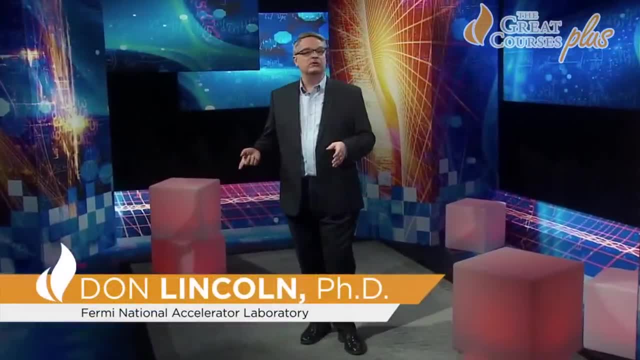 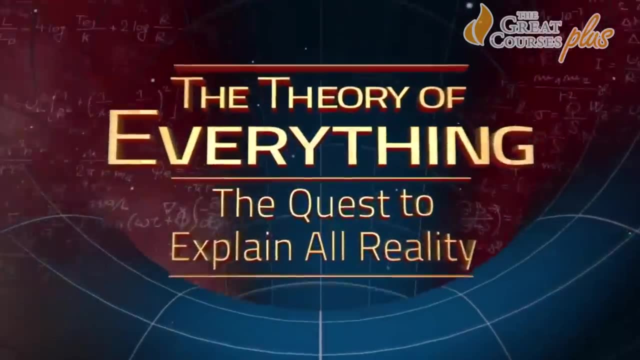 try to emulate At Great Courses. Plus, you can enjoy college-level in-depth lectures not only by Dr Pollack, but also some of the best educators in the world. Some of the other fascinating topics I've enjoyed watching are courses on the elusive theory of everything and the philosophical 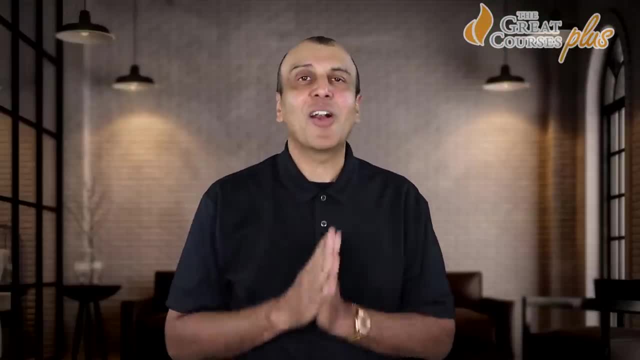 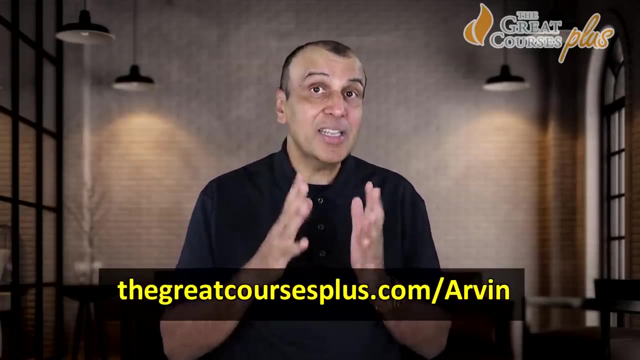 implications of physics. I just love Great Courses Plus and I would be a member regardless of whether they sponsored me or not. It's so easy to sign up because they're offering a special deal right now to Arvin Ashfier's, If you use the link in the description to: 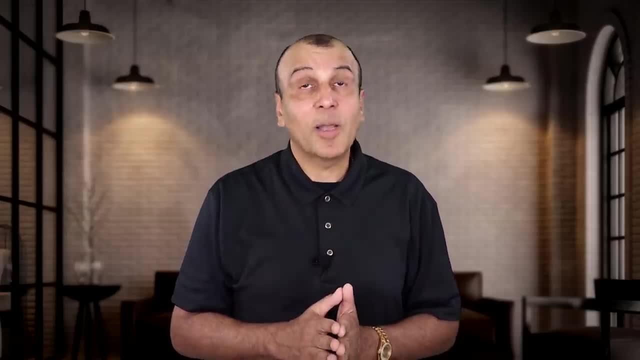 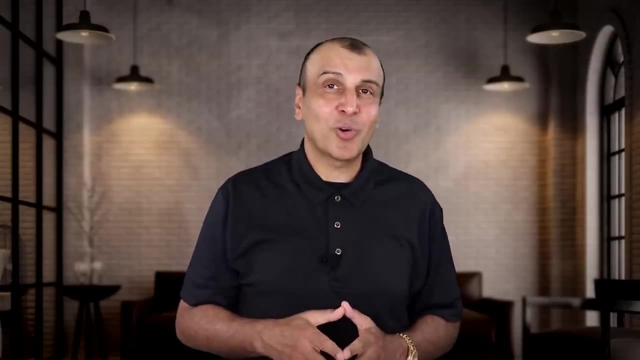 But the universe has no obligation to make sure we feel comfortable about the true nature of reality. This is just one bald ape's opinion about what he thinks are the most important concepts in physics worth remembering, So I hope you found it useful. Now, if you'd like to learn these subjects more in-depth, then you're not going to find. 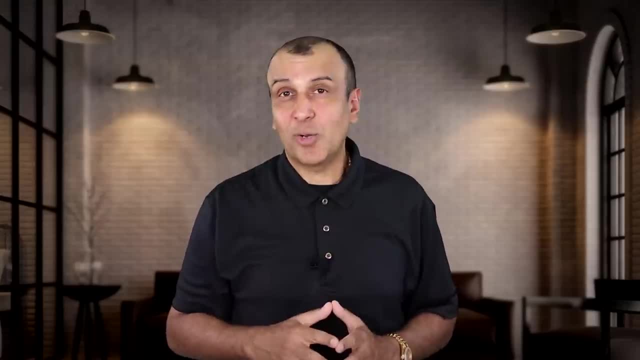 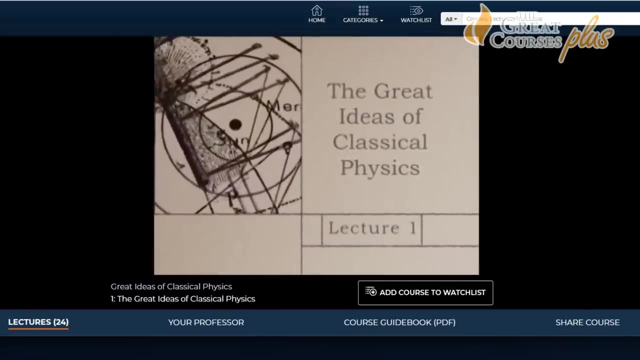 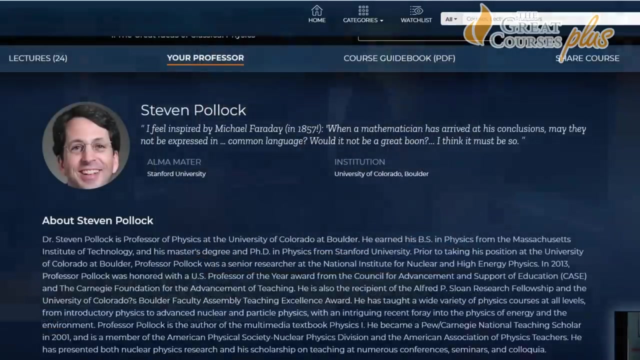 a better on-demand video learning service than that offered by The Great Courses Plus today's sponsor. I was inspired in part to do this video after watching a lecture series called Great Ideas of Classical Physics by Steven Pollack of the University of Colorado, Boulder. His simplicity of language and explanations are models I try to emulate At Great Courses. 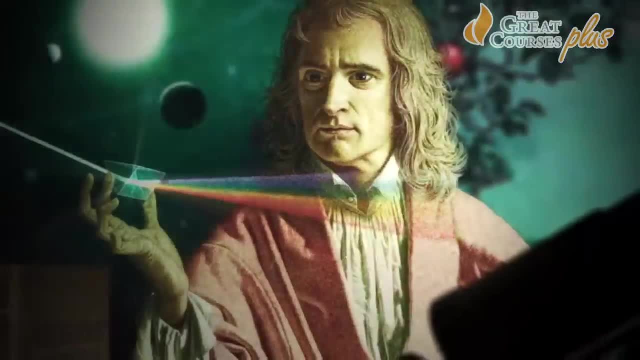 Plus, you can enjoy college-level in-depth lectures. Not only will you be able to learn more about physics, but you'll also be able to learn more about quantum systems- And in-depth lectures not only by Dr Pollack, but also some of the best educators in the. 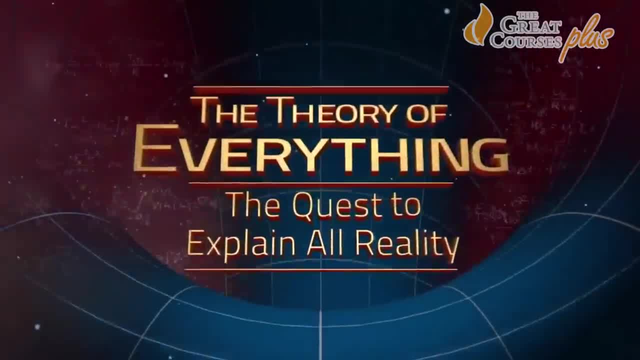 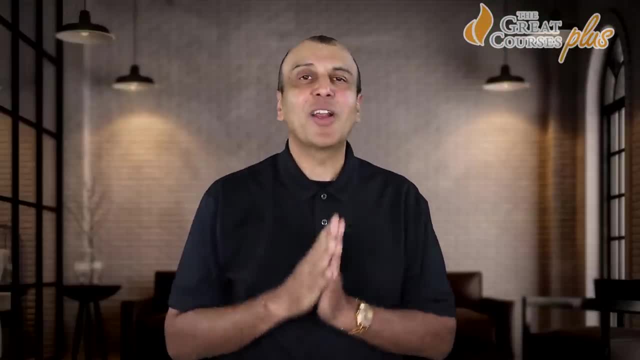 world. Some of the other fascinating topics I've enjoyed watching are courses on the elusive theory of everything and the philosophical implications of physics. I just love Great Courses Plus, and I would be a member regardless of whether they sponsored me or not. It's so easy to sign up because they're offering a special deal right now to Arvind Ashgir. 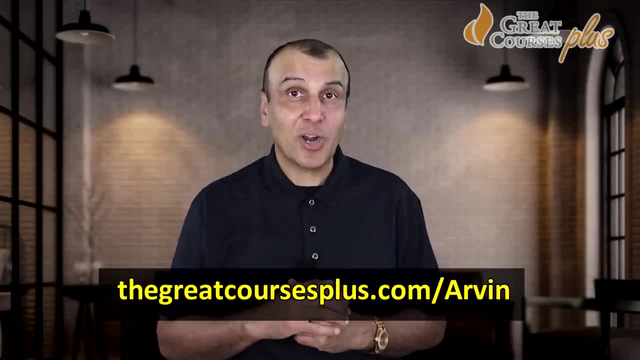 If you use the link in the description, thegreatcoursespluscom forward slash arvind right now you're going to get a free trial, But be sure to use the link in the description. I'd also like to thank my supporters on YouTube and Patreon. I'm going to put the link in the description. 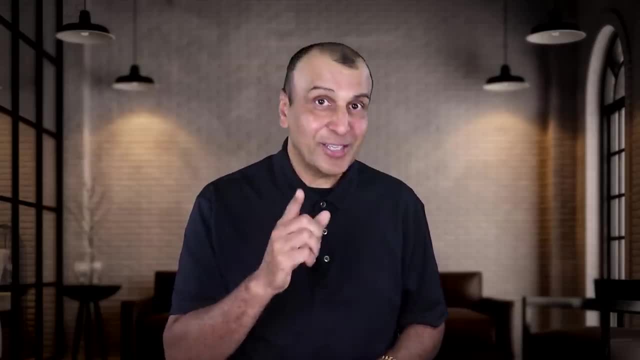 and I'll see you in the next video. If you enjoy my videos, consider joining them. I will see you in the next video, my friend. 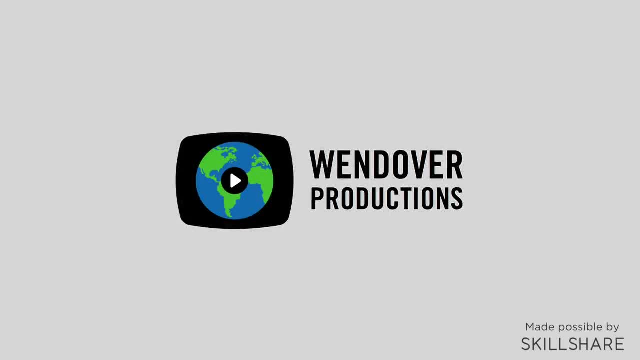 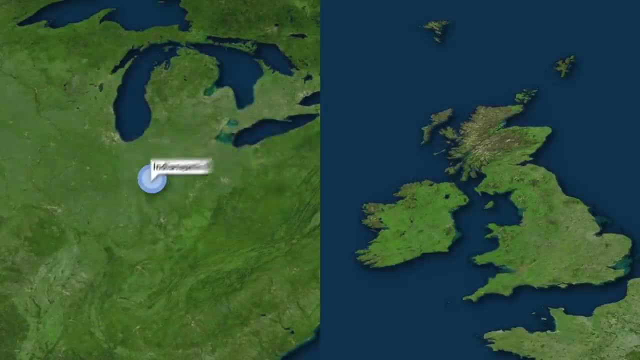 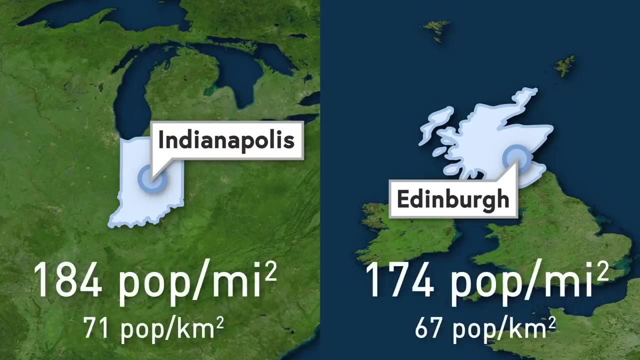 This video was made possible by Skillshare. Learn anything, including how I make these videos for free for two months, by going to sklsh slash Wendover. This is Indiana and this is Scotland. Both have a similar number of inhabitants, a similar size and a similar population density. But here's Indiana's public transportation. 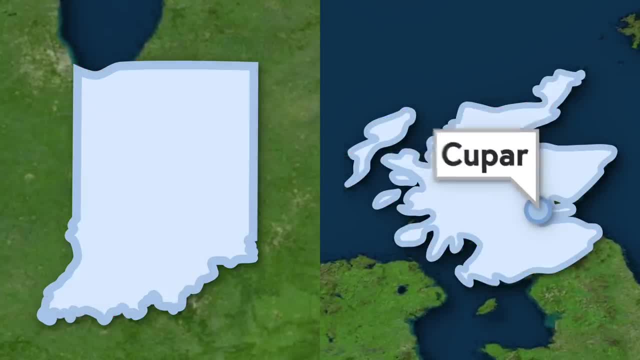 system, and here's Scotland's. You want to get to Cooper, a town of 9,030 miles from the capital. That'll take you 55 minutes on a train that leaves every 30 minutes or an hour, and 40 minutes on a bus that leaves every 40.. You want to get to Anderson, a town.